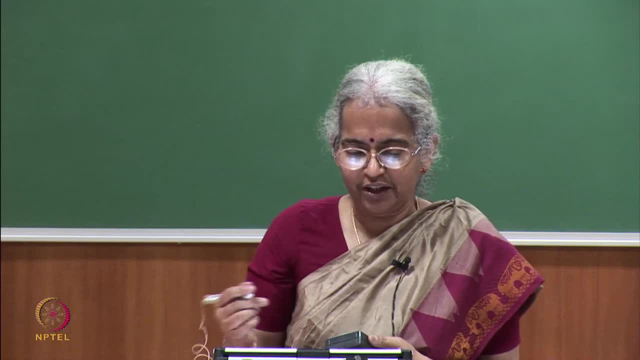 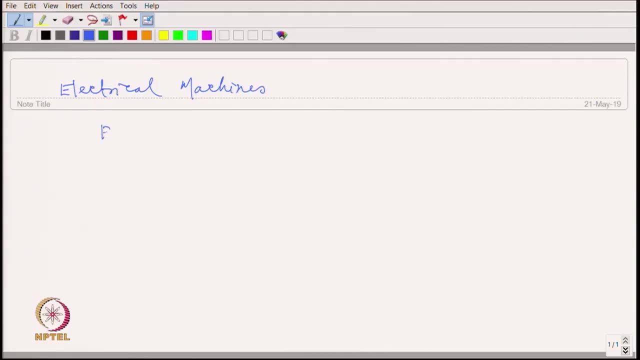 I will go over whatever is the recalling that needs to be done. So if you look at any of the electrical machines, normally they are going to be made up of ferromagnetic materials, Because if you look at electromechanical energy conversion, it is always through a magnetic. 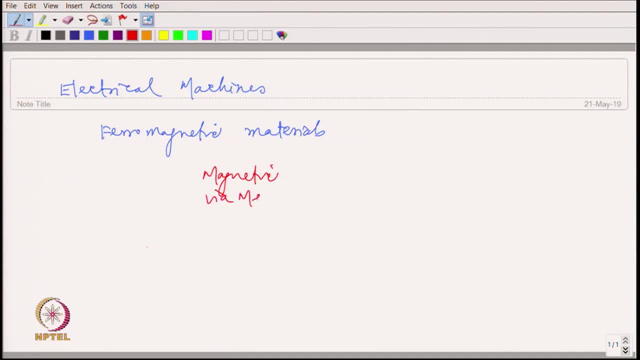 wire media. So I am going to have a magnetic wire media and I am going to have on one side, let us say, electrical energy and I am going to have on the other side mechanical energy. So it is converting from electrical energy to mechanical energy through magnetic wire. 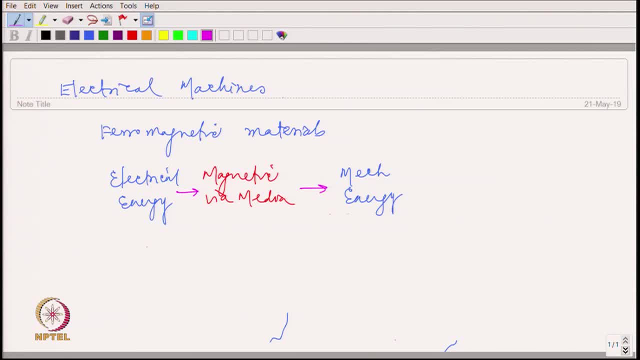 media. So when this is being done, if electrical energy is converted into mechanical energy, it is going to be motoring operation on one side, Whereas if I am going to do from mechanical energy to electrical energy, this is known as generator operation. So I can have either. 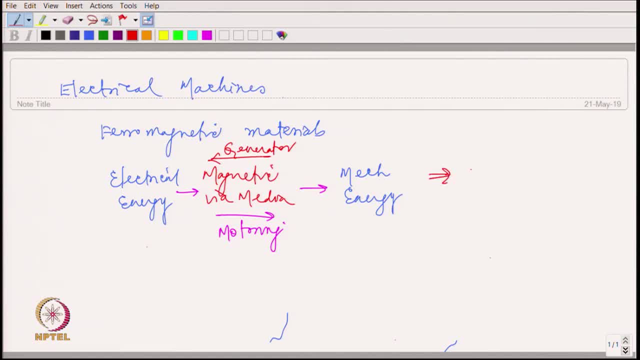 motoring operation or generating operation, The same machine can work as both generator as well as motor. So all I need to do is I have to do the control in such a way, or if I give mechanical energy, it will convert that into electrical energy and it can work as a generator or vice versa. 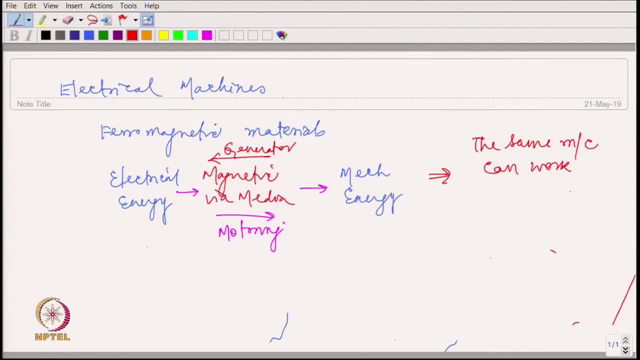 So I can in general say the construction wise and functionality wise. both are almost similar, So the same machine can work as generator as well as motor. But because we are using ferromagnetic material, it is very essential to know about the behavior of ferromagnetic. 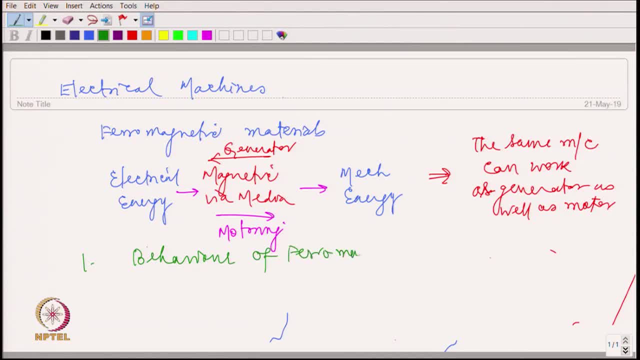 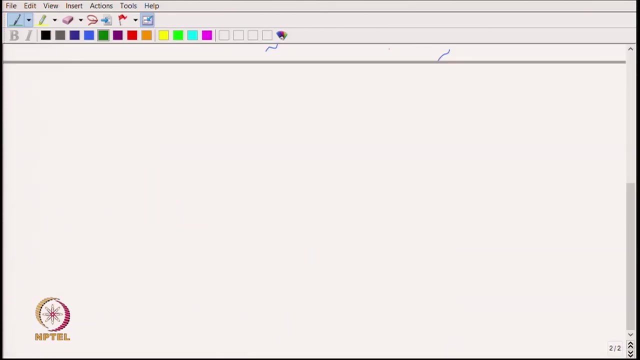 materials, So which we call as basically magnetic circuit. So we call this: whatever is the behavior, we try to analyze it by the help of magnetic circuit concepts. So we will be starting off with this first, Then we are going to look at. so if I actually start the flow of the course, the first and 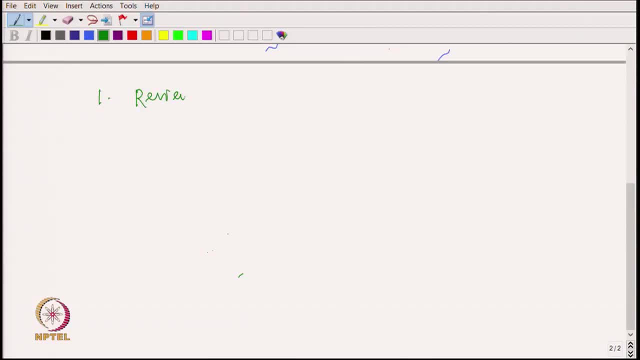 foremost thing we will be doing is review of single phase and three phase circuits. You must have studied this already. you must have seen what is complex notation, what is phasor diagram and how the power is measured and so on. So we will be revisiting these. 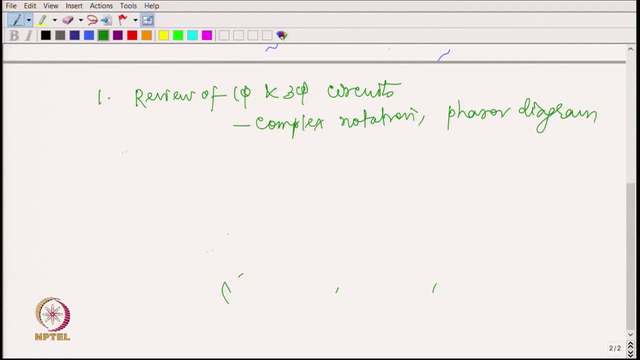 things to some extent. extent first. The second topic is going to be the magnetic circuits. So we will be looking at magnetic circuits as the second topic where we will be talking about the behavior of ferromagnetic material around that- if I wind a wire, how it is going to function. that is what we are. 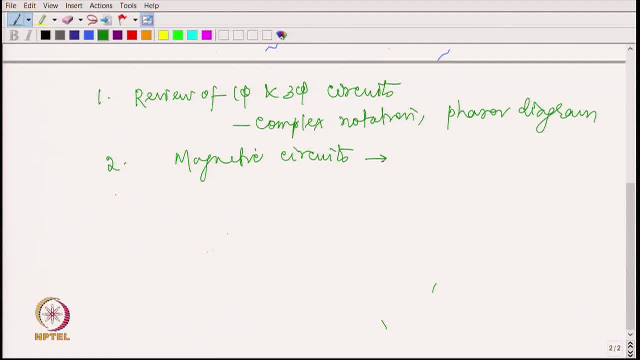 going to look at The third topic after this. we are going to look at basically transformers. So in transformers we will be actually looking at both single-phase and three-phase transformers. We will, of course, start with constructional details: how the transformer is constructed. 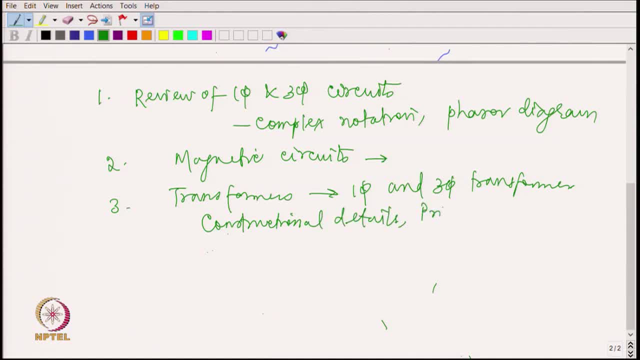 then, after doing that, we will be looking at what is the principle of operation, and then we will be actually looking at the phasor diagram of the transformer, how the voltages and currents are displaced from each other. Then we will be looking at equivalent circuit. 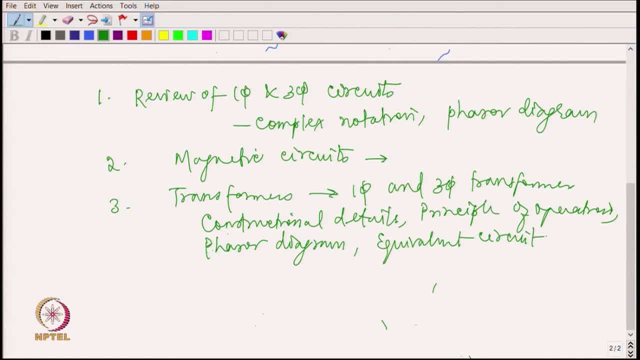 of the transformer. Once we have the equivalent circuit derived, we should be able to really talk about the performance characteristics of the transformers, like voltage regulation and efficiency. These two we will be talking about and after that we will be looking at actually open circuit and short circuit test or testing of transformers from which actually we derive the equivalent. 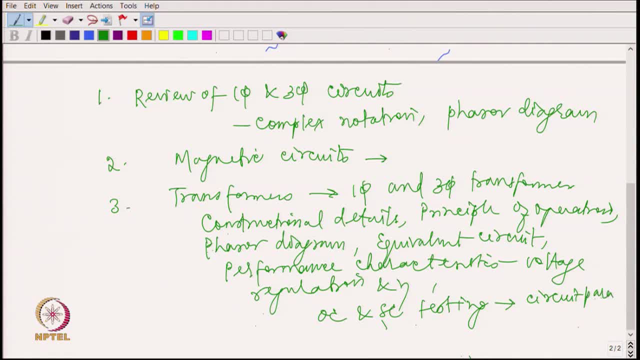 circuit parameters. Then, after looking at these things, we will be actually looking at the auto transformer and instrument transformers, That is, instrument transformers are generally meant for instrumentation, that is, measurements, So we may use potential transformer and current transformer. After looking at all these single-phase transformers, 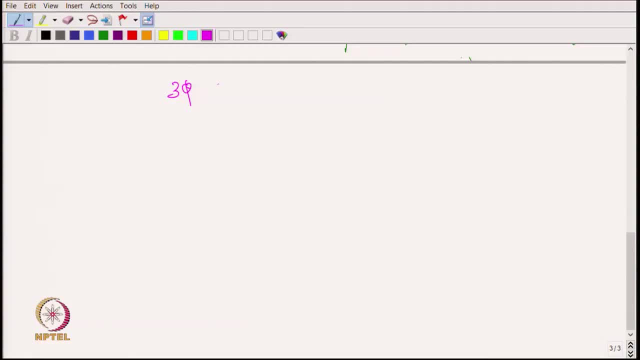 Then we will be going over to three-phase transformers. In three-phase transformers we will be looking at star-star, star-delta, delta-star and delta-delta connection and any other special connections. I forgot to tell you the number of hours. roughly I will. 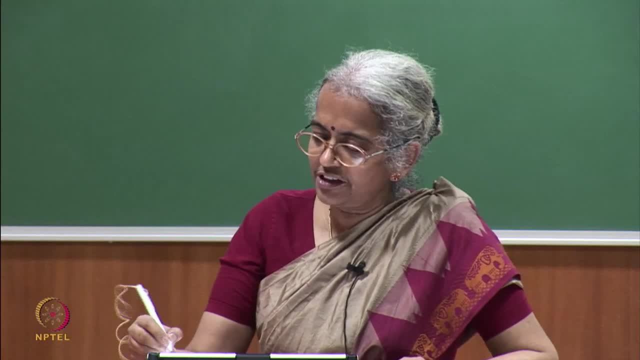 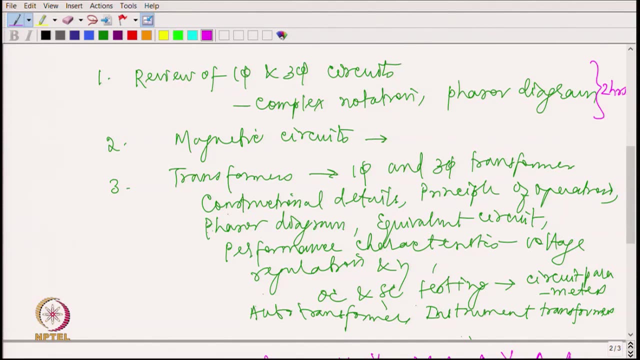 be dwelling on each of these topics. Review of the single-phase and three-phase circuit might take about maximum of 1 to 2 hours, So I am giving myself maximum 2 hours, inclusive of introduction. Magnetic circuit, again, should take anywhere between 2 to 2.5 hours, nothing more than that. Transformers is a vast topic. 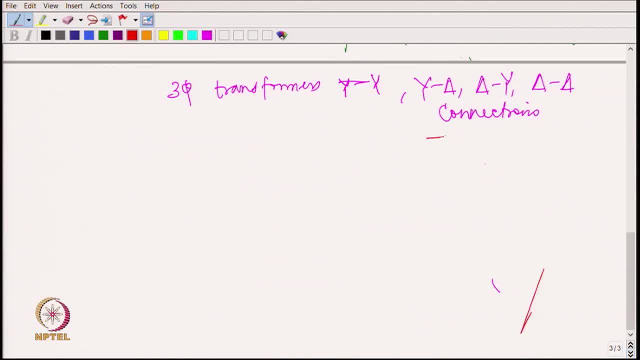 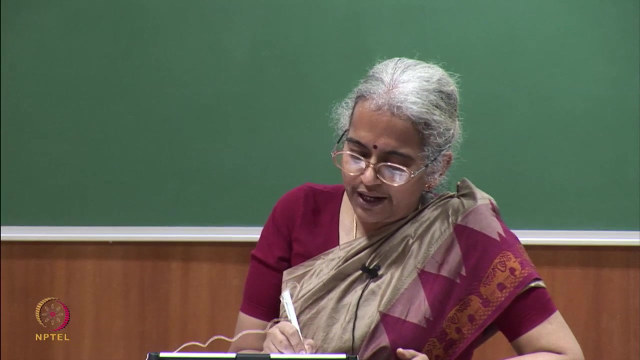 So, inclusive of three-phase transformer, I may be requiring about 8.5 to 10 hours the entire thing. Then the next topic that I am going to have, which is actually the third topic, fourth topic, I suppose fourth topic, The fourth topic actually is going to be the electromechanical. 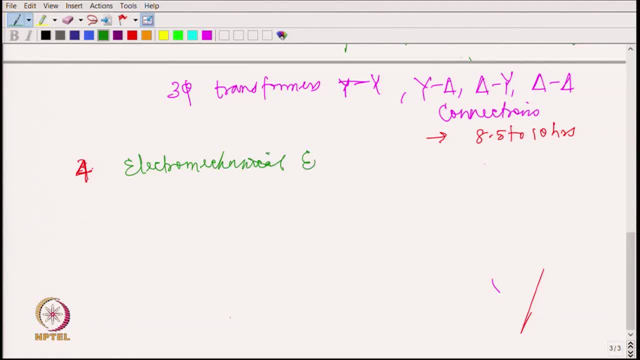 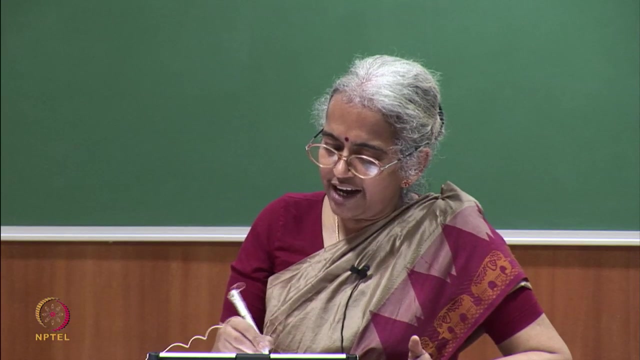 energy conversion principle. Until now, what we had seen in the topic was only static machines. They are not having any moving parts. But if mechanical to electrical energy conversion or electrical to mechanical energy conversion has to take place through a magnetic via media, we have to have definitely looking at energy conversion principles themselves. So this: 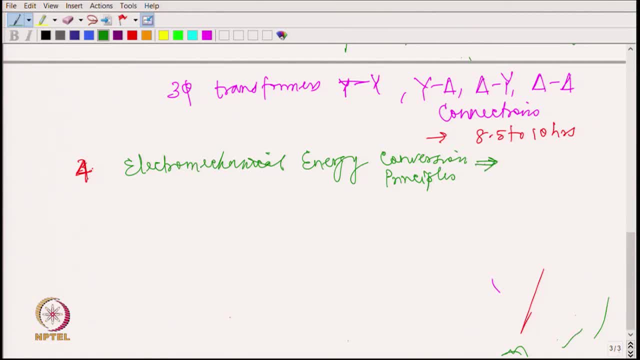 is just giving an introduction to how electromechanical energy conversion takes place. This will take anywhere between about 2 to 2.5 hours- 6.7 hours. After this, we will be looking at DC machines, because this is one of the simpler machines. 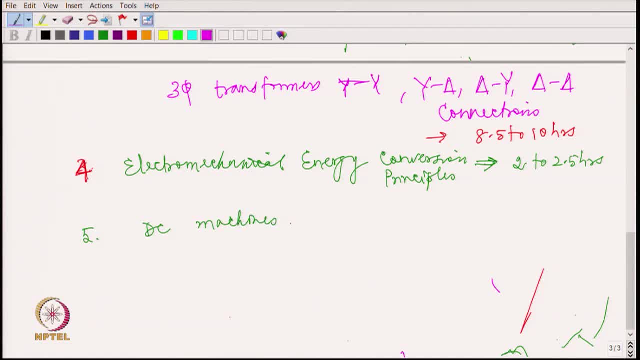 in terms of operation. I would not say constructional principle, definitely in terms of operation. So we will be looking at first of all basic construction, after that we will look at the classification of DC machine working principle, Then after that we will be looking at something called armature reaction. 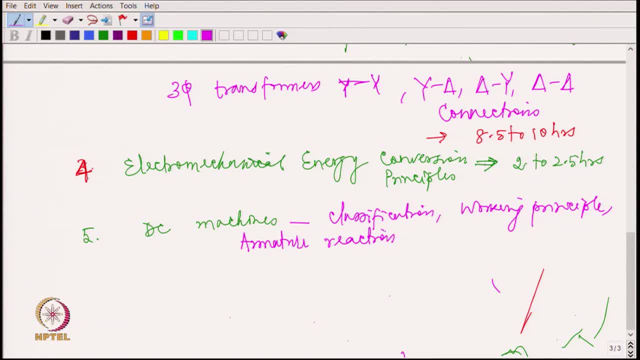 What happens when the armature is also creating some flux along with the field, So this is known as armature reaction. Then we will be looking at characteristics of the DC machine. So if I am talking about motor, I have to talk about speed, torque characteristics. 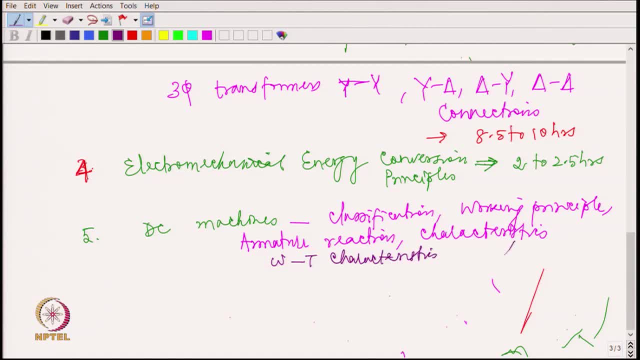 If I am talking about the generator, I should talk about voltage versus current characteristics. So this we will be looking at. Then, when we are talking about motor, we will be actually concentrating on starting- how we start a DC motor. Then we will be looking at braking very briefly and we will also be looking at speed control. 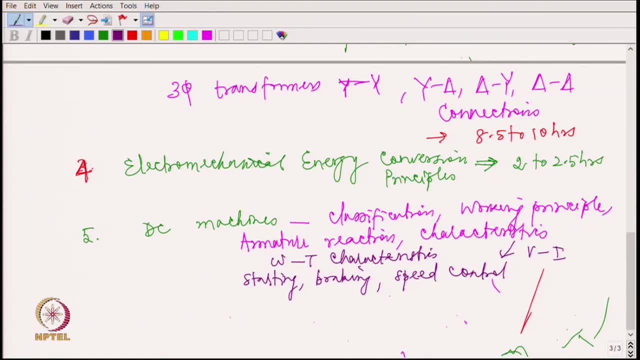 How to control the speed of a DC motor. These are the different things we will be looking at. Of course, I have left out testing of DC motor. Okay, For testing of DC machine. we should actually look at the testing of DC machines as well. 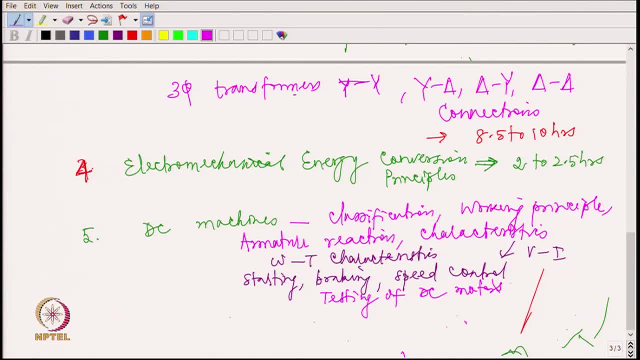 Depending upon, of course, time availability of time. Then, after completing DC machines, we will be actually taking up induction machines, which is one of the most important AC machines. If you look at the industries, 80 percent of the electrical energy actually is used. 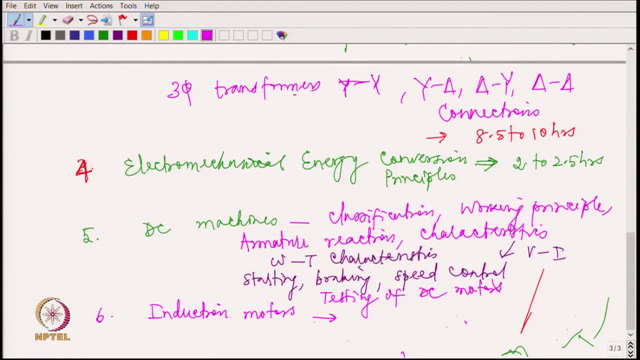 in factories or industries is consumed by induction motors, three-phase induction motors. So we will be first looking at three-phase induction motor. In three-phase induction motor we will be looking at construction. but even before that we should look at revolving magnetic field theory. 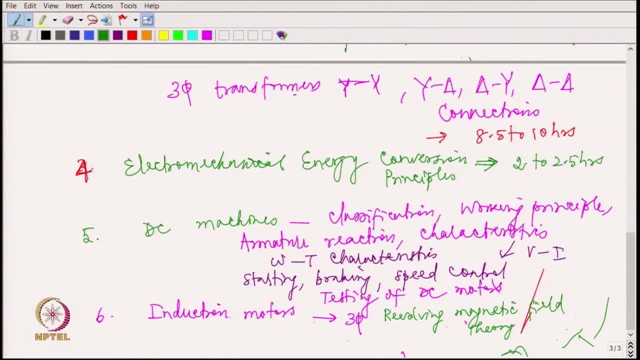 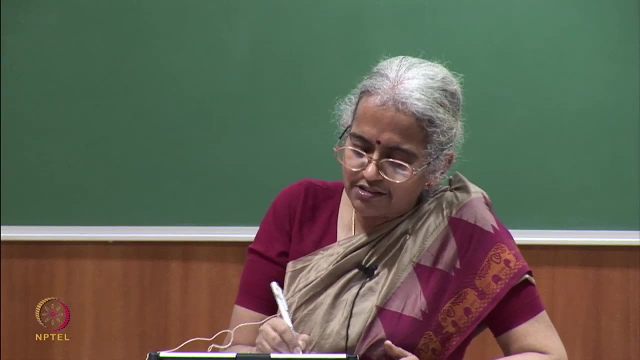 How we are going to have, when three-phase voltages are applied to three-phase time, displaced phase, displaced winding. How are revolving magnetic field theory? How are revolving magnetic field is created? This is how we will start the three-phase induction motor. Then, in the three-phase induction motor itself, we will talk about construction, two types. 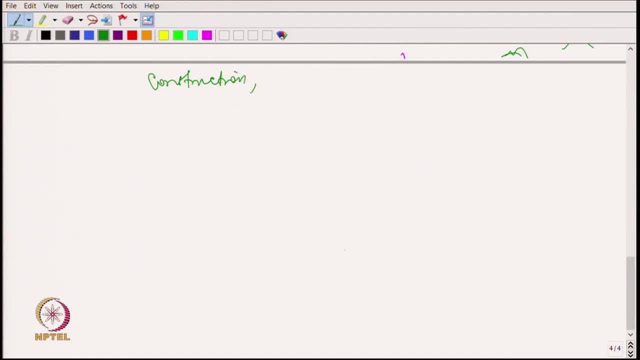 of construction, that is, scroll cage and wound rotor. Then we will talk about principle of operation. After looking at the principle of operation, then we will be looking at phasor diagram and equivalent circuit. Okay, Okay, Okay, Okay. After looking at the equivalent circuit, we will be able to derive the torque expression. 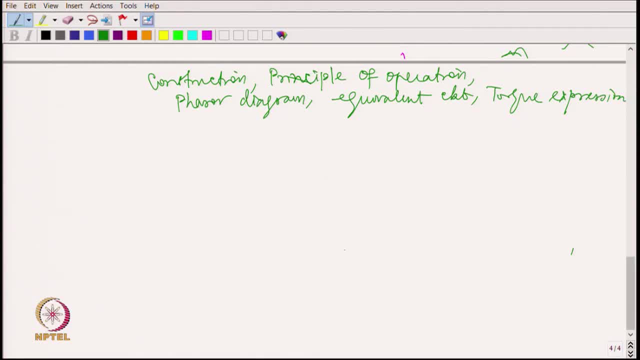 torque slip or torque speed characteristics, Then we will be clearly looking at how the characteristics are dependent upon these expression. So we will be talking about the speed torque characteristics mainly. Then. after that we will be looking at starting. what are all the different starting methods? 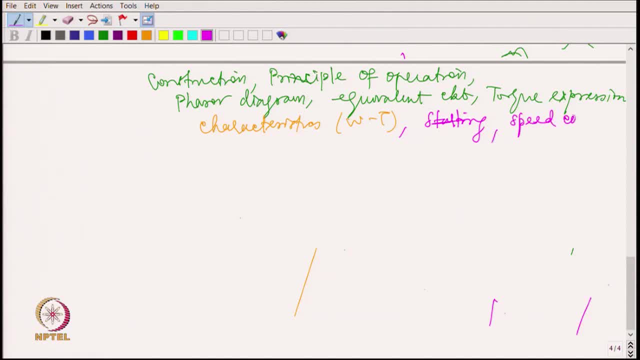 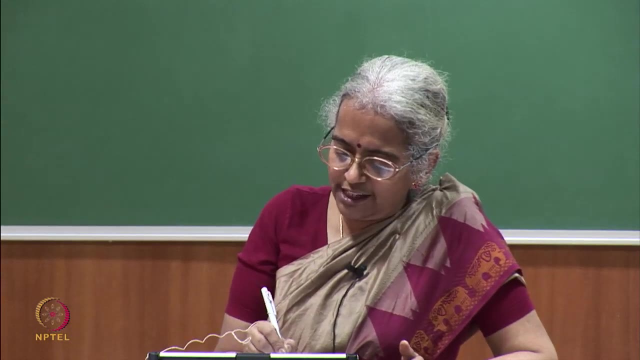 Okay. Okay, Then we can look at speed control and very little bit about braking. So these are the topics that will be covered under induction motor. Then, if time permits, we will also look at single-phase induction motor. Let us see how it goes. 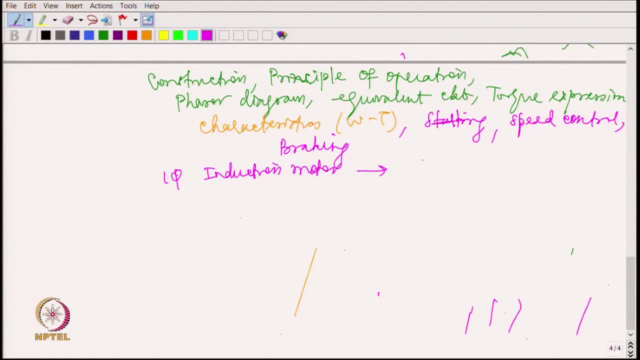 So, single-phase induction motor, we may be looking at basically double field revolving theory, Okay, And then we will be looking at again equivalent circuit characteristics etc. So these are going to be different topics in single-phase induction motor. I would not like to call this as a separate topic because this will be pretty small. 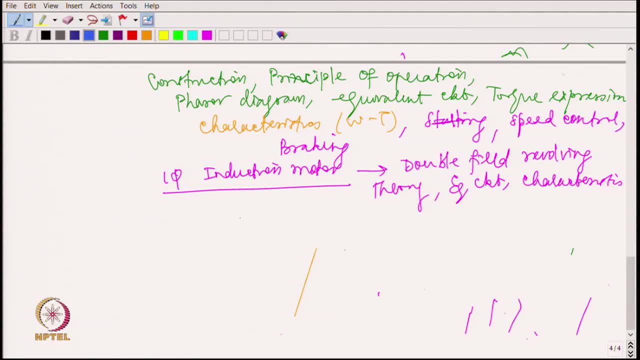 So for three-phase induction motor, I might take anywhere between, again, 8 to 10 hours minimum. This might take about 1 to 2 hours, because we are just going to touch upon this, nothing more than that. Then the next topic that we would be looking at will be synchronous machines. 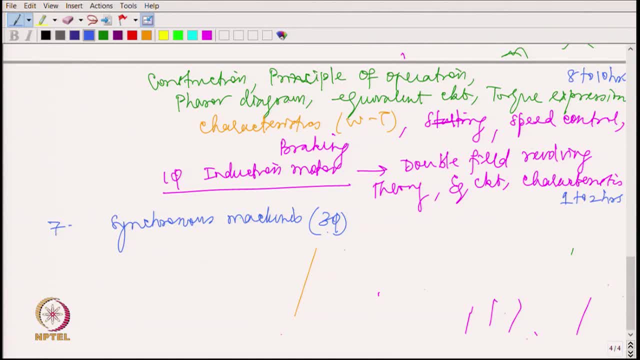 This is also a three-phase machine, but we will be concentrating on this as a generator, So we call a three-phase synchronous machine. Okay, So synchronous machine working as a generator, as an alternator. So we will be looking at alternator and its working basically in this particular topic. 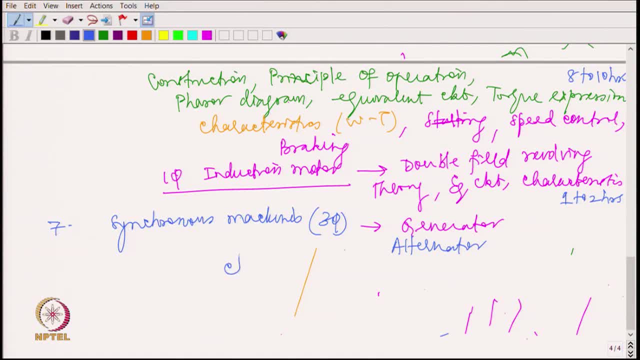 The synchronous machines generally. we will start with classification, Then we will look at construction. After looking at construction, here we will be concentrating more on the winding arrangement. So we will talk about something called winding. So this is called winding factor and how it influences the voltage generation in a synchronous 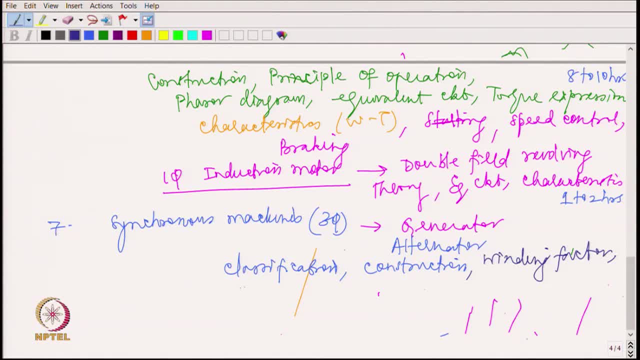 machine. After that we will be looking at power angle relationship and equivalent circuit. And because it is working as a generator, it is very important to look at VI characteristics of the generator, Whether it will be able to maintain a constant voltage in case of disturbance. how do we handle? 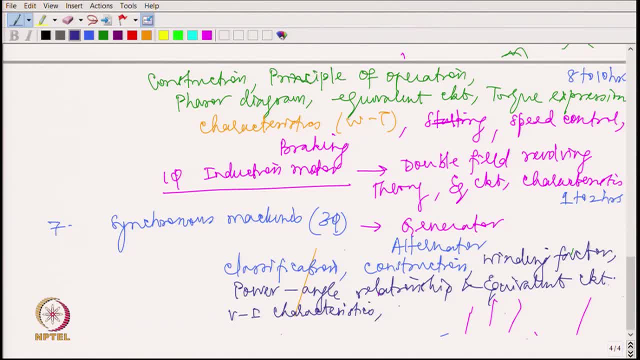 it. These things will be talked about After this. we will be talking about power factor control, which is one of the most important aspects of the synchronous machine. Then we will be talking about the same machine functioning as a motor. very briefly, that. 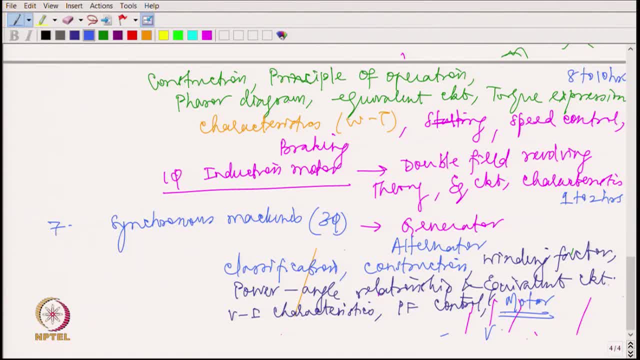 is synchronous motor, under which we will be talking about V and inverted V characteristics. Okay, Okay, Thank you. One more thing I have forgotten: we also need to look at the generator as how it can be synchronized, how the synchronization can be done with the three-phase grid. 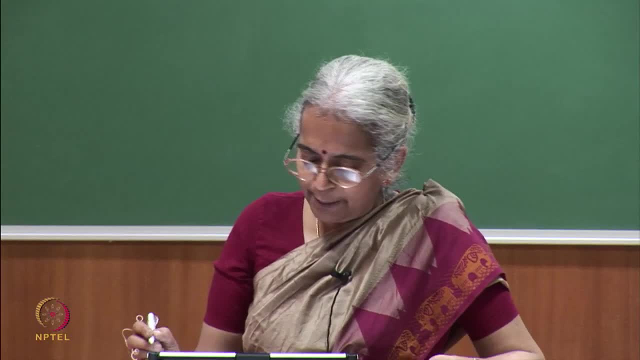 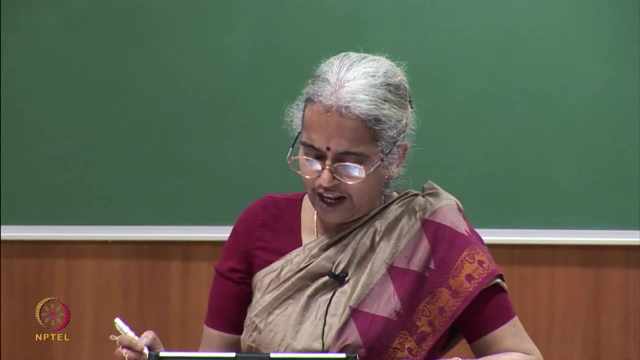 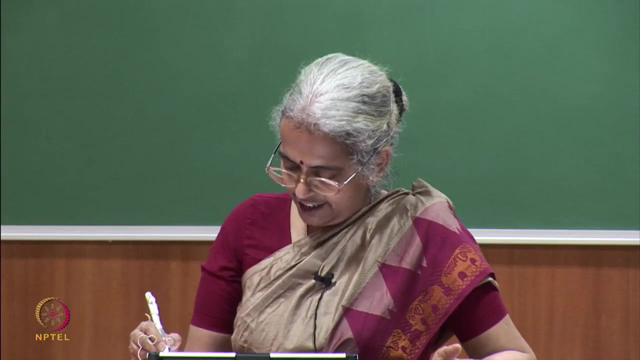 So this is an important thing we need to do when we want to feed power from the synchronous generator into the three-phase grid. So we will be talking about synchronization as well. Okay, In my opinion, this should not take as long as what it has taken for induction machine. 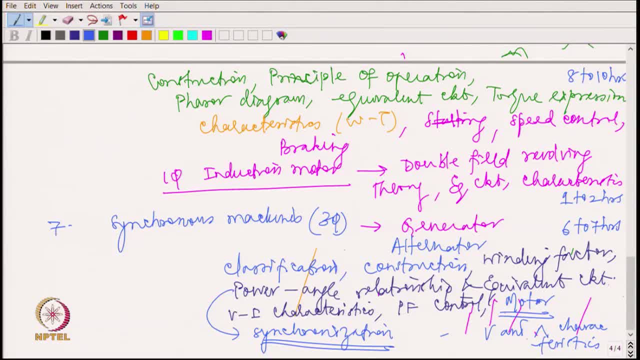 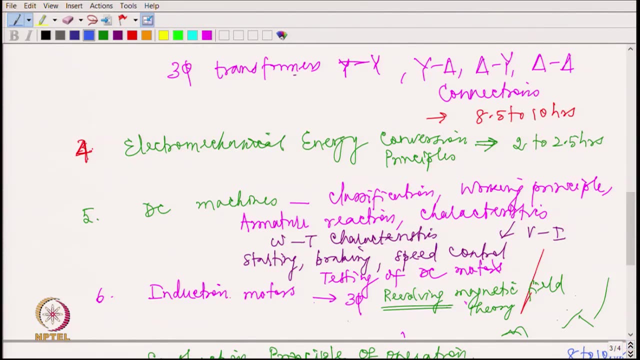 So it may be anywhere between 6 to 7 hours. So I think on the whole, if we actually compute the total number of hours, we will be spending about 6 plus 2, 8, 8 plus 8, 16 and we are having electromechanical energy conversion. 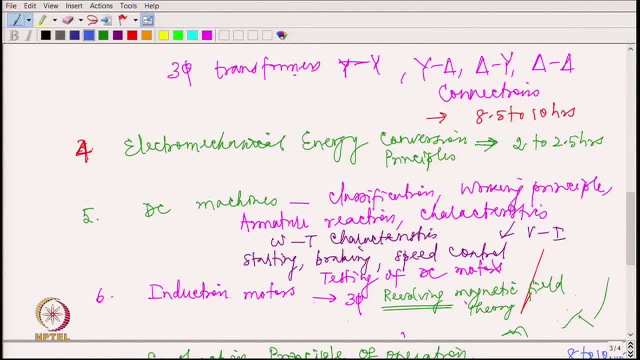 principle plus transformers May be about 2 hours. Okay, So we will be spending about 10, 12.5 hours. So 16 plus 12, 28 have a leftover DC machine. I have not given any time here that has to. 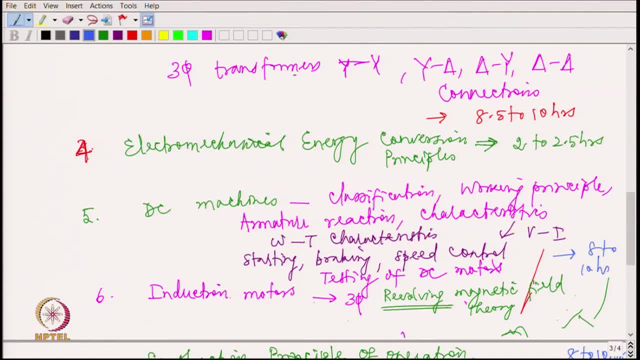 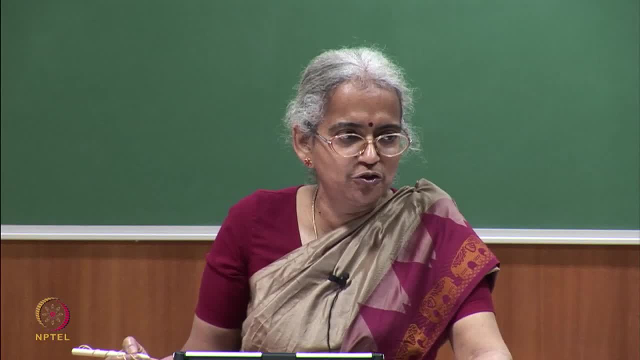 be about again 8 to 10 hours, So about 38 hours or 36 hours gone. here, then introduction and review everything together, about 2 plus 2, 4 hours, So I think it comes to about 40 to 42 hours. 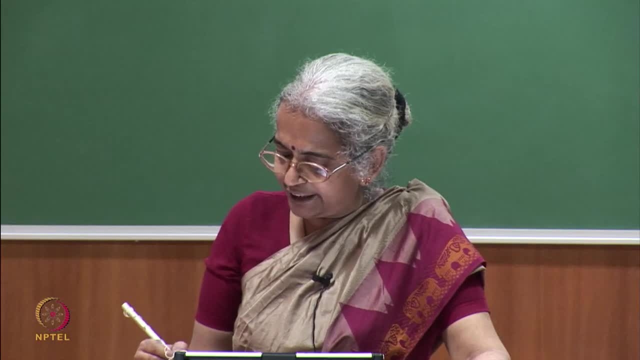 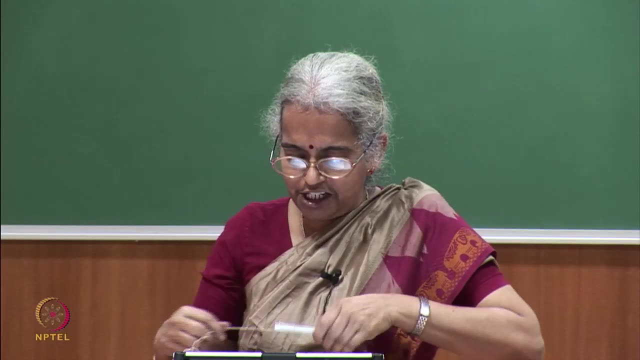 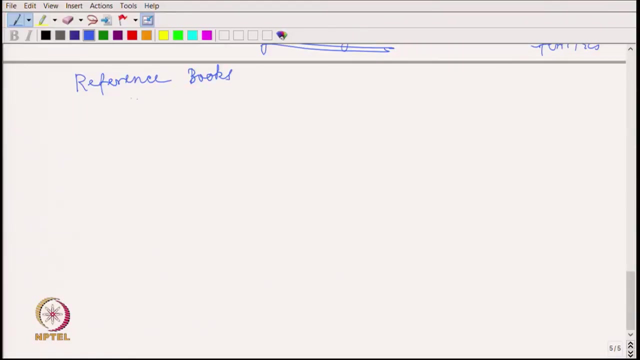 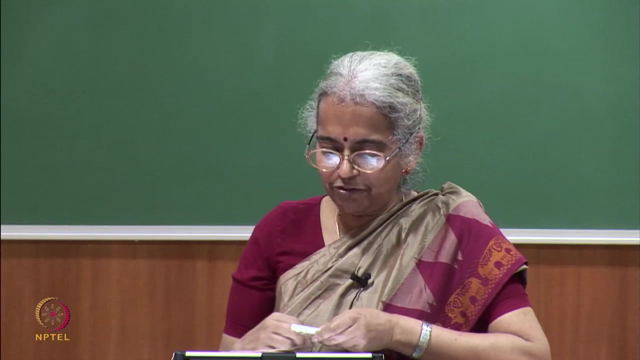 So that is the way the entire lecture is going to be planned. Okay, We have some reference books for this electrical machines course, So let me write them out. I would like to start with simplest of books, basically for electrical machines, Although some of the topics I mentioned may not be covered very well in this book. nevertheless, 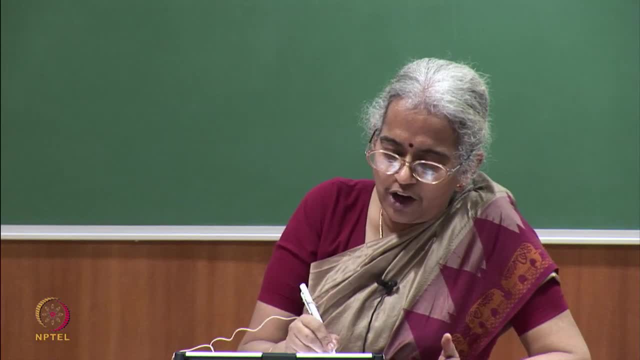 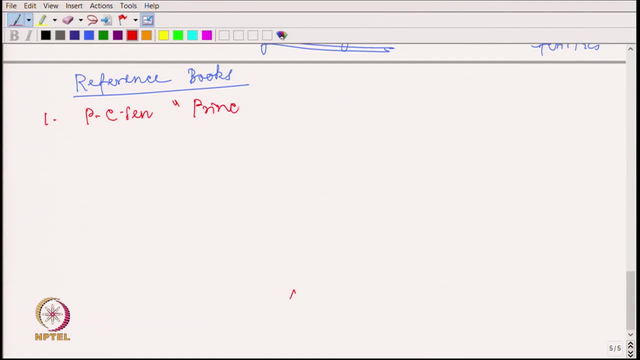 for a beginner it is very, very easy to read that book, So I would rather recommend that book. This book is very easy to read. The book is written by P C Sen And this is called Principles of Electrical Machines and Power Electronics. 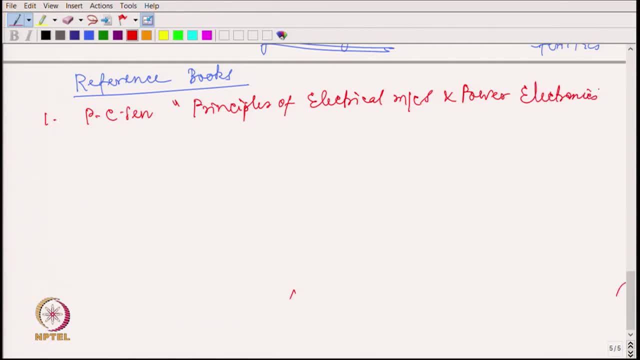 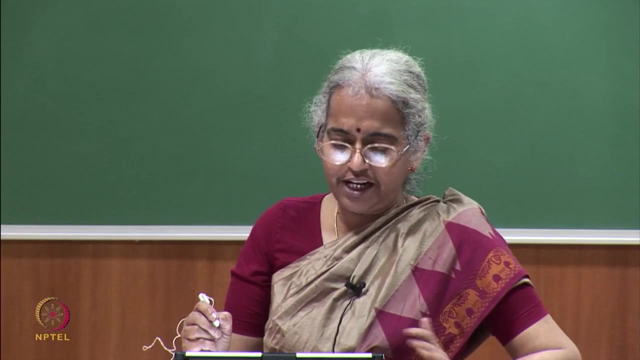 Of course we will not be going into power electronics portion, no doubt. But this covers electrical machines from a fundamental principle. It starts with magnetic circuits and so on. there are appendices given on three-phase circuits and single-phase circuits. So I think it almost gives you a very good introduction to entire machines course. 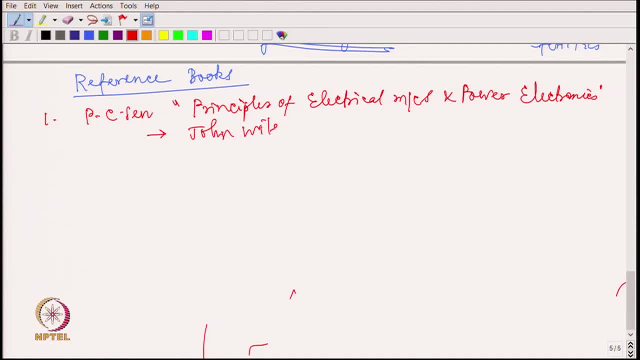 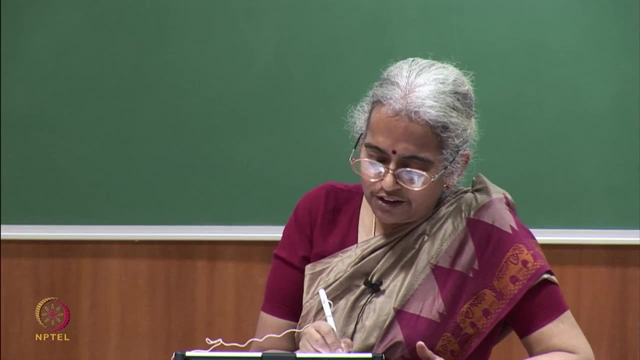 This is from John Wiley and second edition is available as far as I remember. If you ask me the year, I do not remember. The second book I would rather recommend very strongly is that there is one book on DC machines. Let me probably erase it. 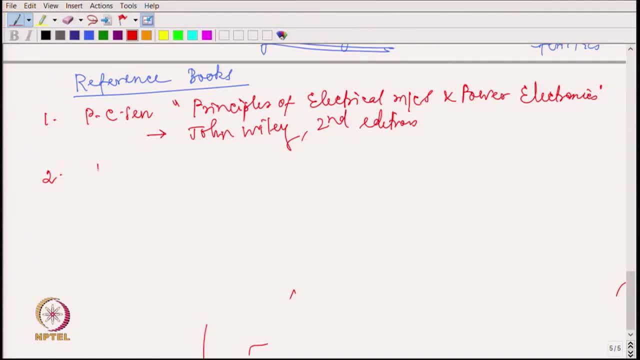 Let me write in the same order as I have done. Okay. So M G Say and O Taylor. there is a book on DC machines by these two people. It is a vast book. that is why I would not give this as a principle reference book. 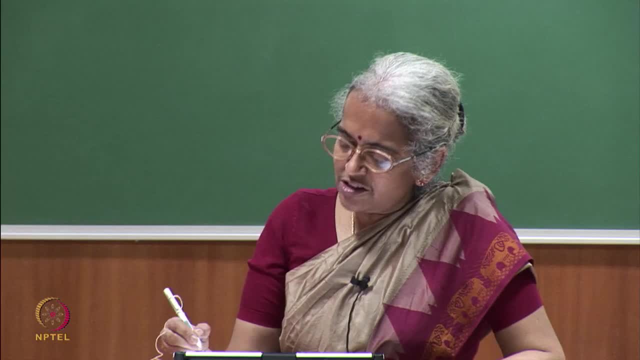 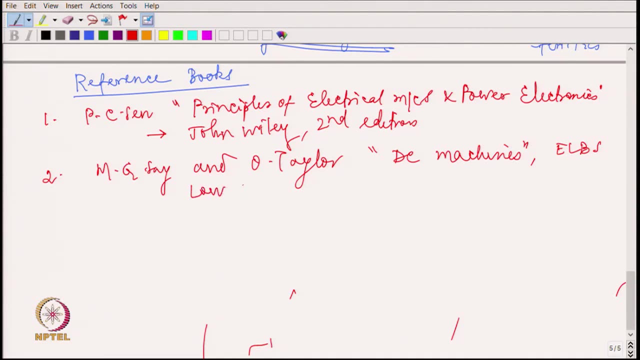 But it is written extremely well and this is from probably ELBS. it used to come from ELBS, English Language Book Society, low price edition. I do not know whether Pearson has taken it already. I am not sure. Similarly, the counterpart in the AC side is again by M G Say. 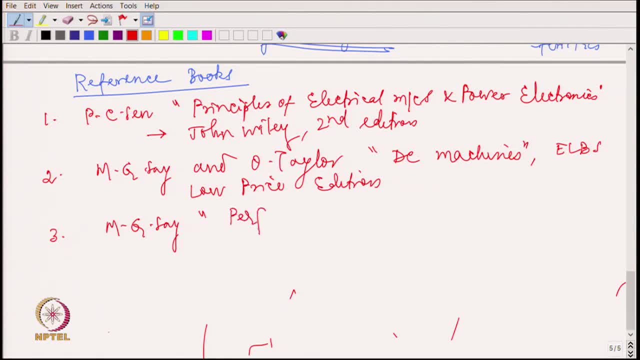 This is actually performance and design of alternating current machines. This is again a very vast book, But it is a very good book, But the explanations are extremely good and this is also from ELBS. this is a low price edition. Then I would say one more book which is really worthy of reading, that is by Fitzgerald and 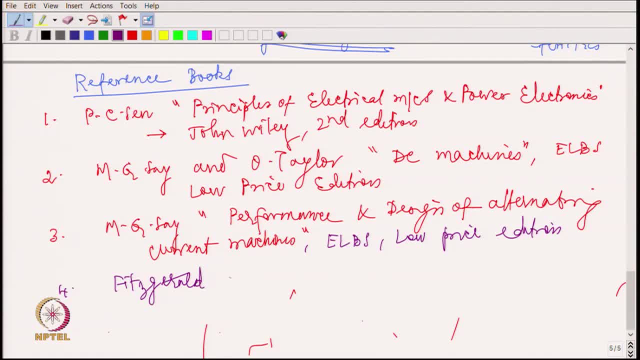 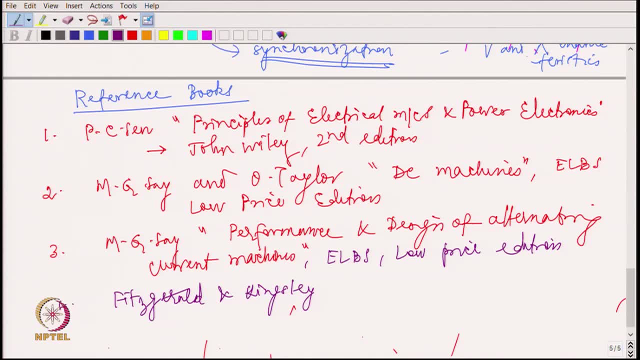 Kingsley. Of course there is a third author, Oman's. I have left him out. He is a great author, He is a great author, He is a great author, He is a great writer, He is a great writer. 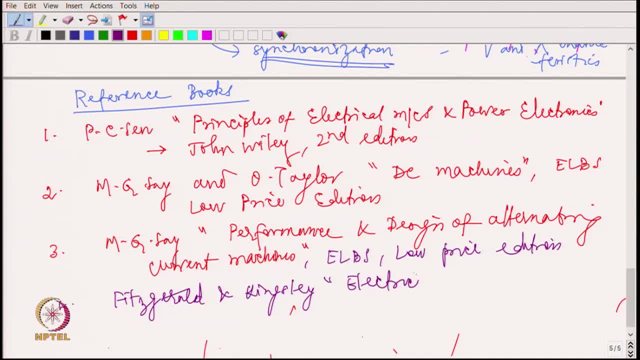 He is a great writer, So this is actually electric machinery. I think 7th edition. something has come now, as far as I remember, And this is from McGraw Hill. There are definitely other books that are available as well, from Pearson, for example. 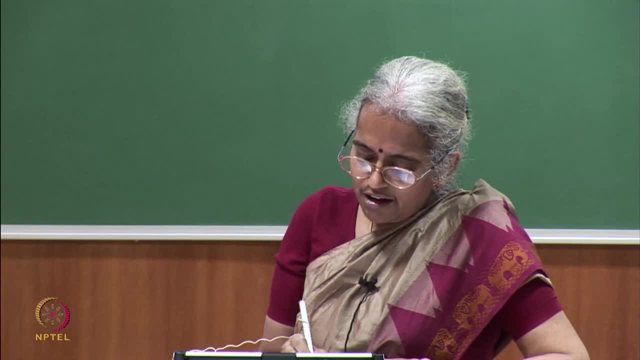 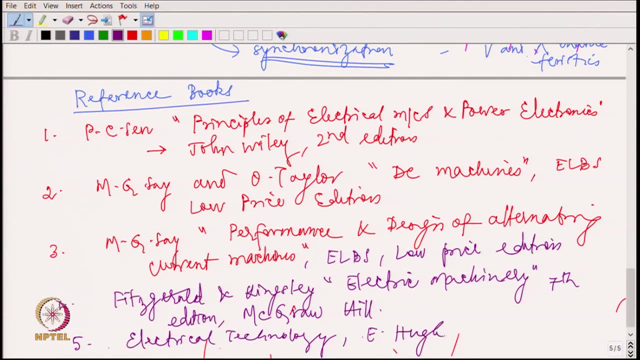 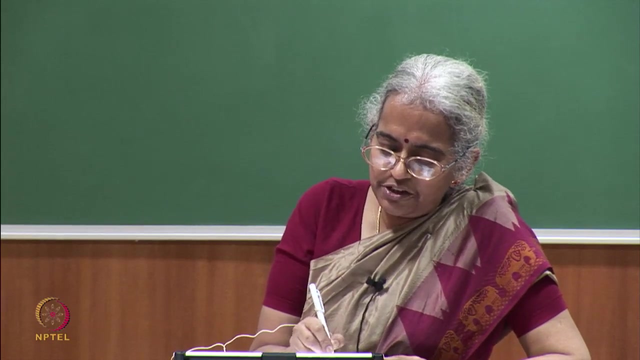 there is electrical technology by Dewey. This is a book by Dewey. This is a book by Dewey. This is an article by Dewey: Edward Hughes. this is a very good book. there is one more which is actually Electric Machinery. 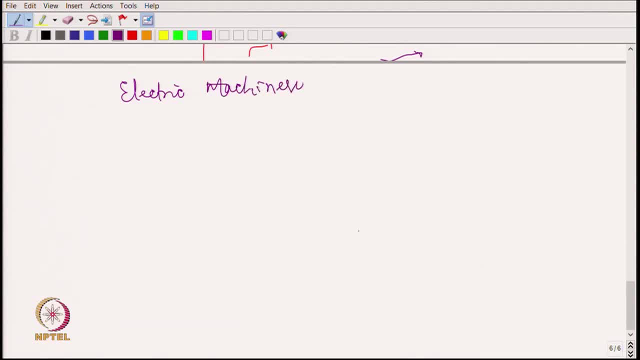 by Chapman, Stephen Chapman- these are from Pearson and one more Indian author book, probably Electric Machinery by, or Electrical Machines by, Nagarath and Kothari. I think this is from Tata Meghra Hill. it used to be from Tata Meghra Hill, so this: 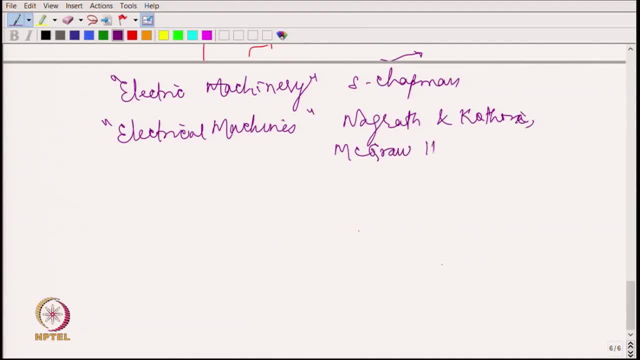 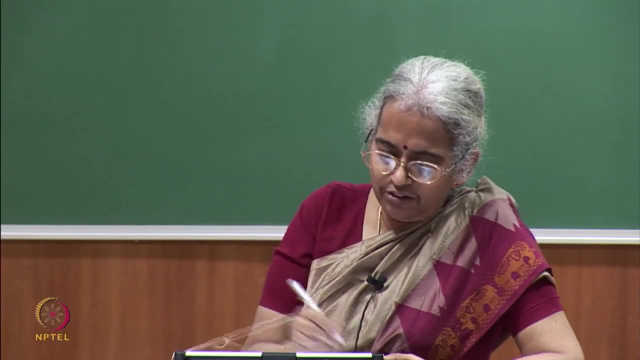 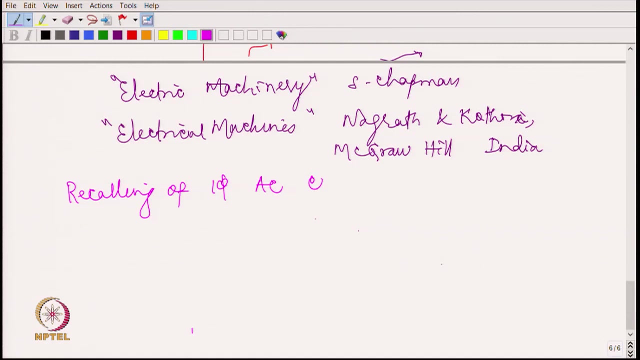 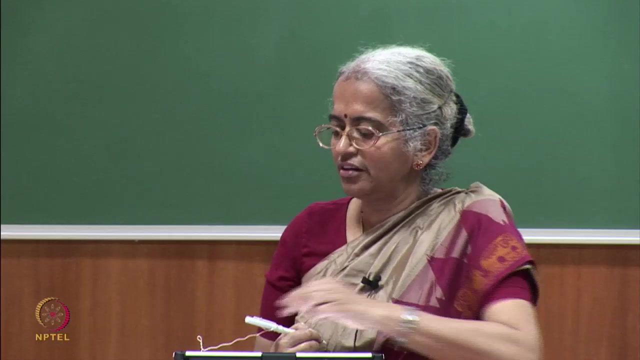 is now Meghra Hill, India. So these are some of the reference books that we might like to refer to whenever we have some confusion in any of the topics. So let me start with actually the Recalling of single phase AC circuits. So I am starting with recalling single phase AC circuits. all of you guys know that generally. 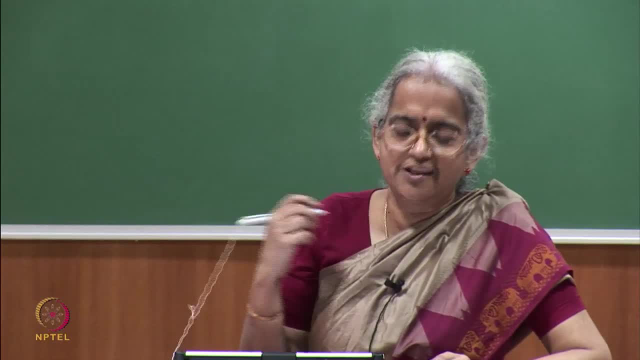 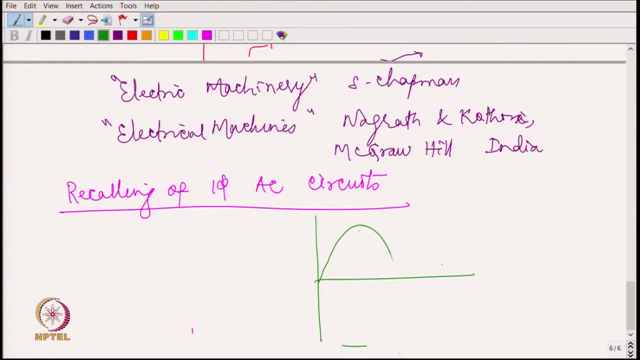 when we talk about single phase AC circuit, we are going to have sinusoidal excitation basically. So we are going to give basically a sinusoidal excitation. what we mean by excitation is a voltage. We are going to give a sinusoidal voltage. 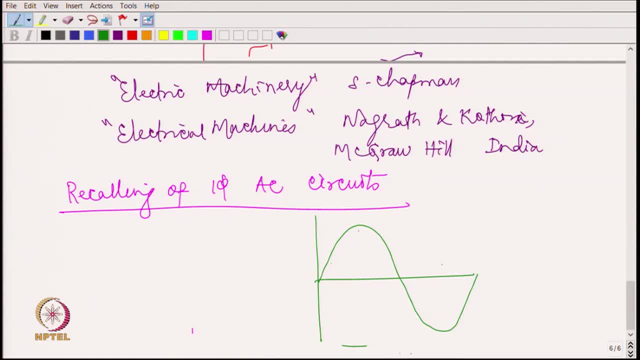 So whenever we have a sinusoidal voltage, rather than using that as a sign quantity, let us say this is T. if I am writing this with respect to time, I have to add and subtract sinusoidal quantities, I have to multiply, I have to differentiate, integrate. all of them needs. 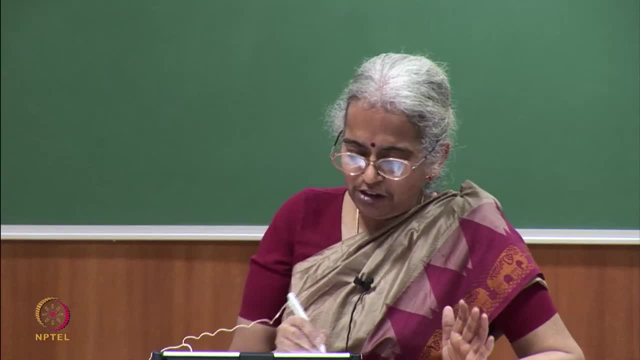 to be done on this sinusoidal quantity, Because I am sure fundamental elements are there. I have to add and subtract sinusoidal quantities, I have to multiply, I have to differentiate, integrate all of them. needs to be done on this sinusoidal quantity. 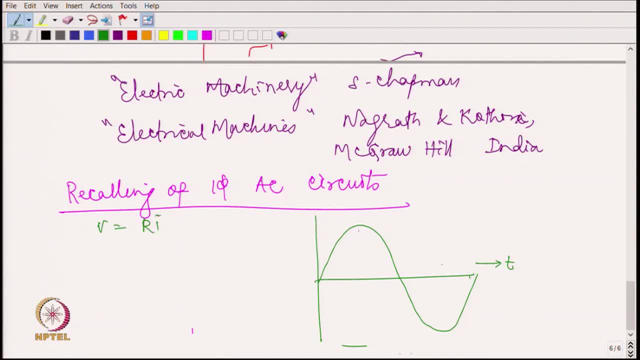 So I am going to write this in an electric circuit. you guys know So V equal to Ri. this is corresponding to resistance. I can write L, Di by Dt equal to V. this is with reference to inductance C, dV by Dt equal. 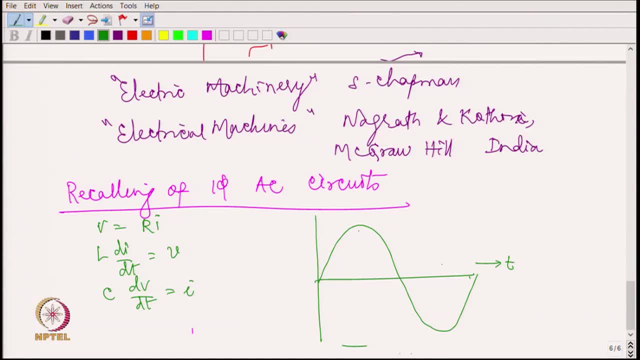 to current. this is with reference to capacitance. So you can very well see that I have V and I without being differentiated or integrated here. And ultimately, if I want power, I should say V times I- right, instantaneous power. So I will have to multiply some of the sinusoidal quantities I have to differentiate some of 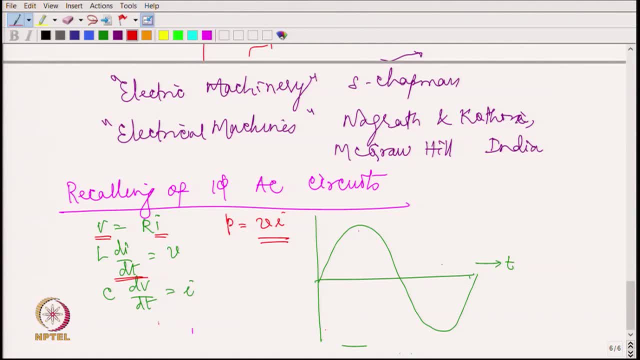 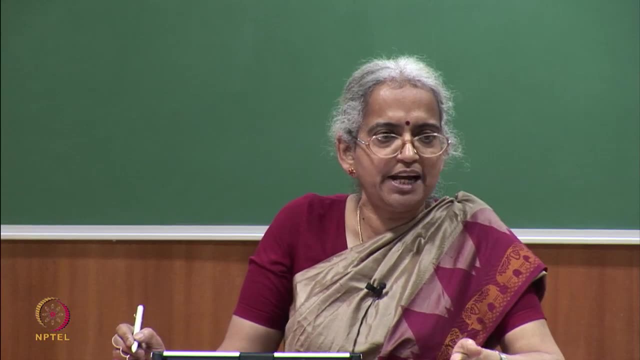 the sinusoidal quantities I have to integrate if I want actually voltage equal to 1 by C integral Idt right. So I have to integrate these quantities. The major advantage of using a sinusoidal quantity is that whether you differentiate, whether you integrate, whether you multiply, whether you divide, you are going to get ultimately. 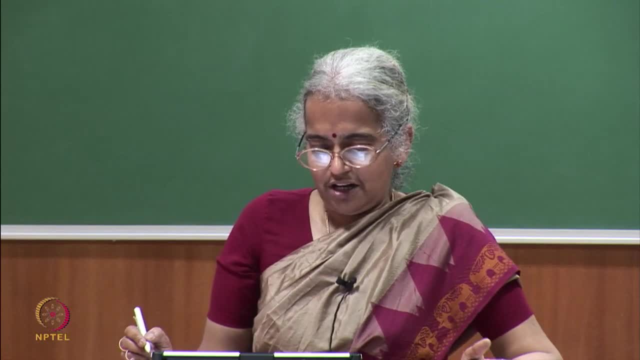 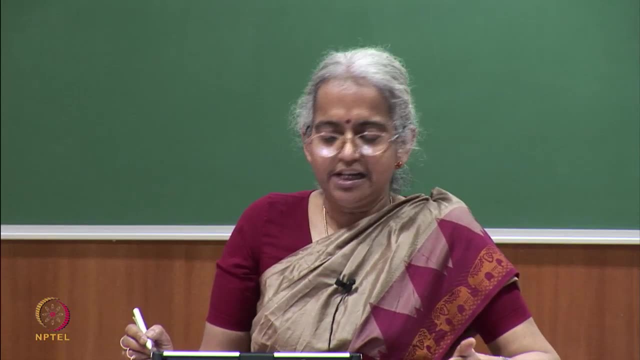 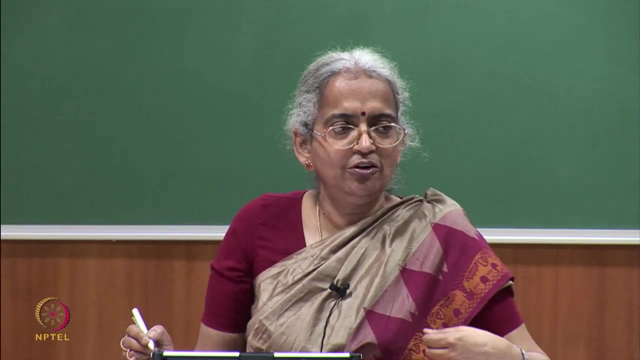 sinusoidal quantity itself And in nature, most of these waveforms that are available are sinusoidal in nature, So that is the reason why and it does not have any abrupt rise or fall, and in nature nothing grows abruptly, nothing really. you know, maybe death is the only thing which. 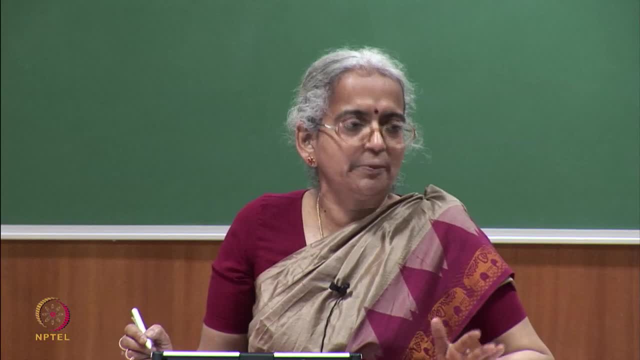 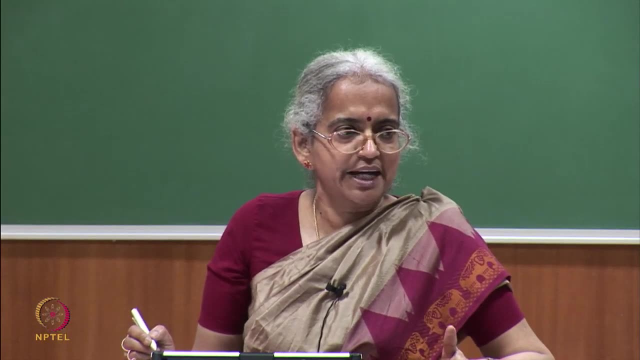 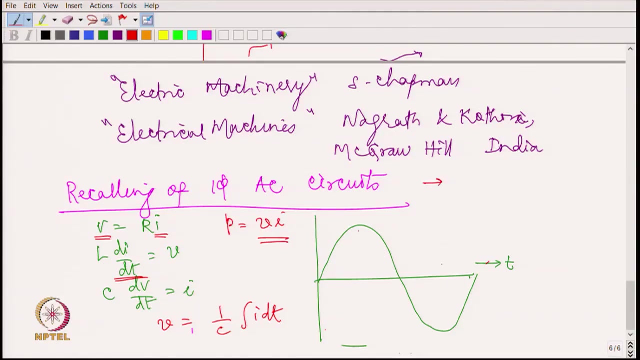 occurs abruptly, But other than that, everything is not. you know, It does not happen Right, It does not happen abruptly. That is the reason why we are using sinusoidal quantities in all our electricity and magnetism. Now, if I have to actually refer to this quantity in the form of a vector or rotating vector, 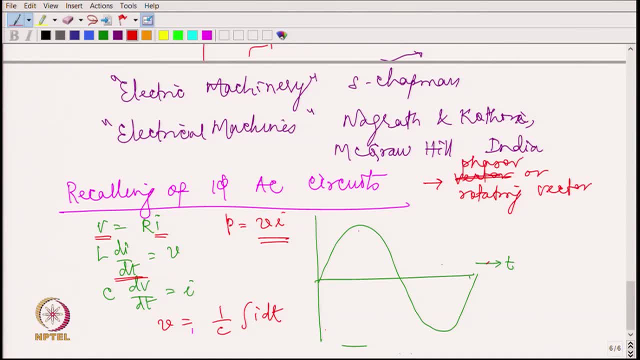 Actually rotating vector is generally known as phasor. So if I want to refer to this as a phasor, Then what I can do is I can try to look at the projection along this axis and try to plot it. For example, I am looking at time t equal to 0, at that point I am having 0 value. 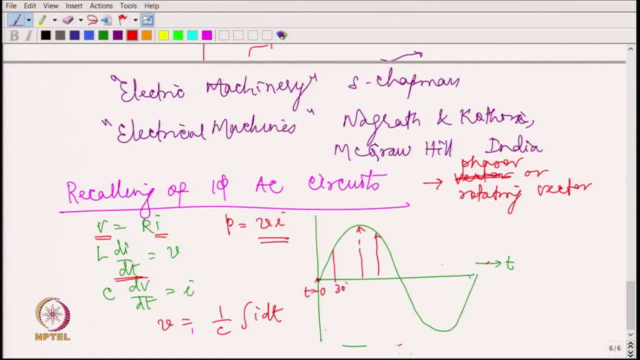 If I look at corresponding to, say, 30 degrees- point, this is 30 degrees- I am going to have half the value of the peak. So I can actually project this as though a vector is rotating continuously with respect to time. So when I had time, t equal to 0, if I actually specify this vector somewhat like this: 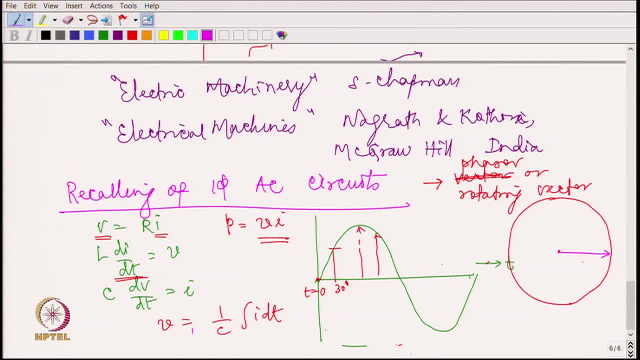 If I look at the vertical projection, or projection along the vertical axis, the magnitude is 0, which corresponds to the sinusoidal quantity, also at time t equal to 0. When I look at 30 degrees, I can just take it along. maybe it would have rotated exactly. 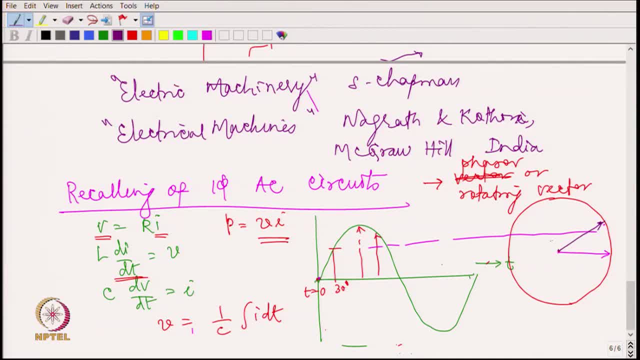 by 30 degrees here, And this is actually 30 degrees. Okay, And if I call this point as a, this point is going to correspond to a. So if I try to look at the vertical projection, it will exactly have this value. 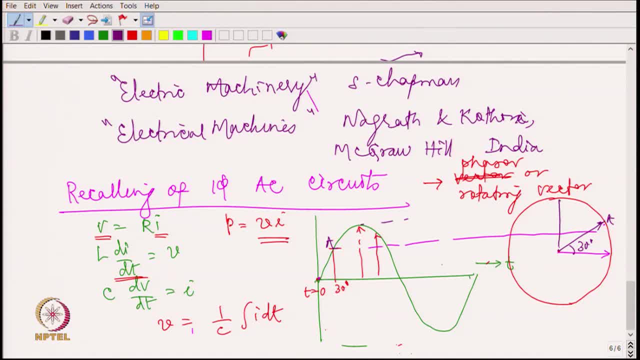 So, similarly, I should be able to draw: basically this corresponds to 90 degree, this corresponds to 180 degree and this corresponds to 270 degrees and this corresponds to 360 degrees again. So if I say that this is actually oscillating at a 30 degree angle, 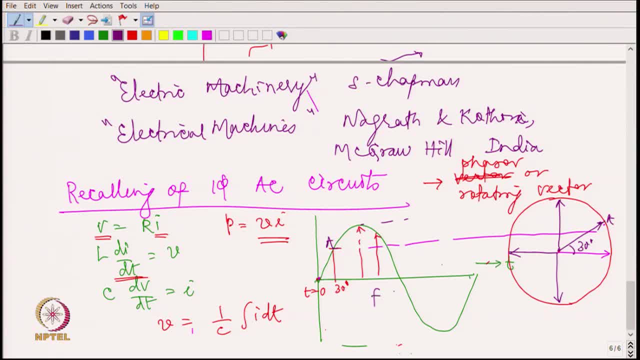 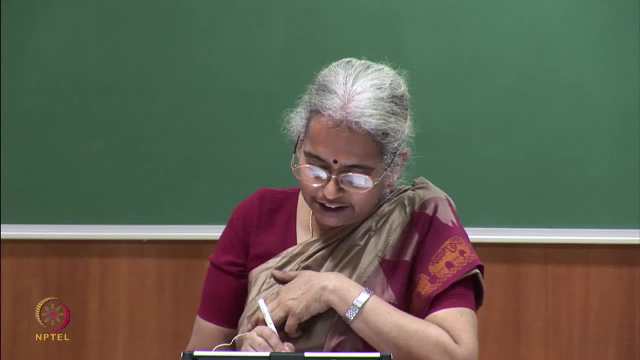 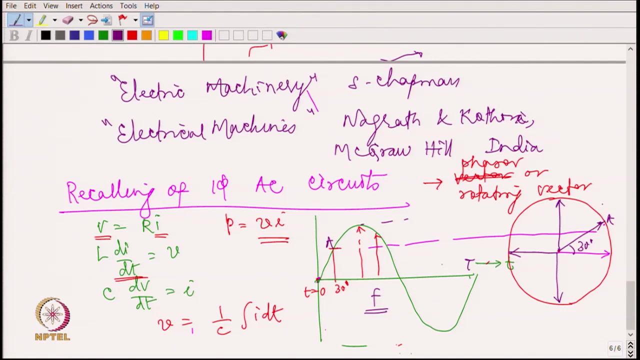 Okay, This is oscillating at a frequency of f in 1 second. I am going to see f such oscillations. So if I am traversing from 0 degree to 360 degrees completely, or if I go from small, that is, 0, to capital T here, then I would have traversed this by 2 pi radians or 360 degrees. 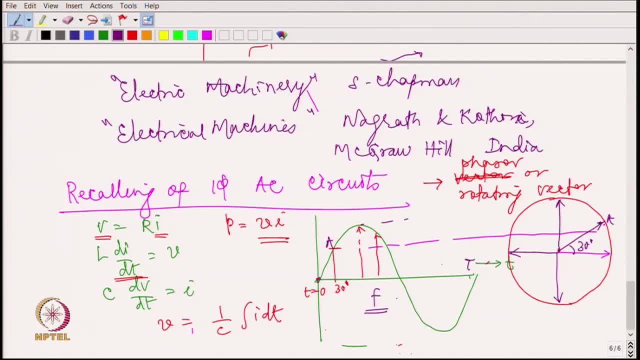 So if I am saying that f times it is going to oscillate in 1 second, I will have 2 pi times f as the radians that is traversed within 1 second. So this is the angle that is traversed in 1 second. 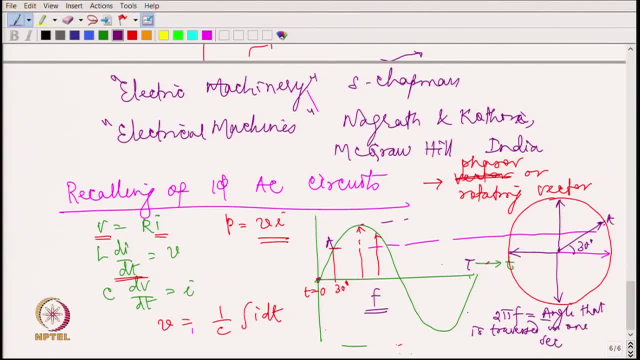 So we call this as angular velocity, which is omega. So we are going to say this as omega equal to 2 pi f. So when we are plotting with respect to angle, we can write this as omega t. Okay, Okay, Okay. 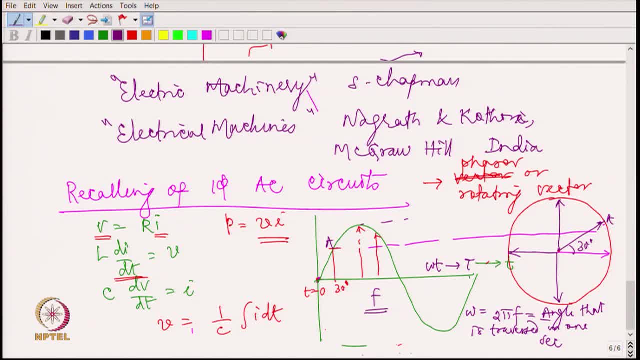 Okay, Okay, Okay. So this is the angular velocity rather than t, Because I can say 2 pi f is the angular velocity, So 2 pi f times t will be the angle that is traversed. So every time when we draw actually the waveform of voltage or current, we will always write: 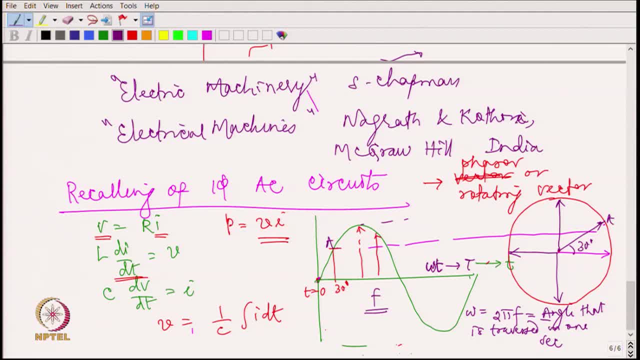 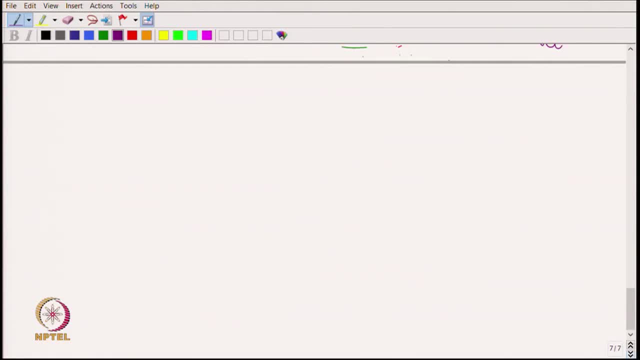 the angle. write the x-axis as omega t rather than t. This is what we are going to do Now. if I am having 1 inductance, probably let us say L di by dt, equal to VL voltage across the inductance. Let us say: 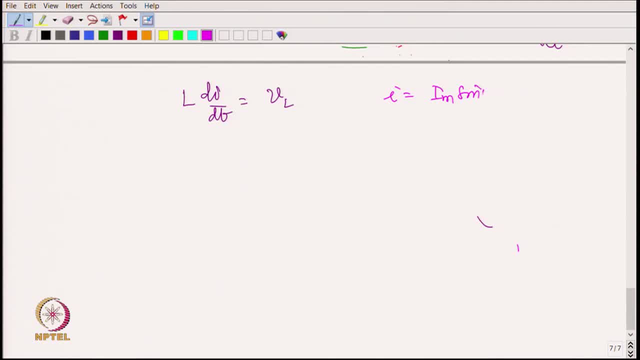 I am going to have I equal to some Im sin omega t right. So if I do that, I am going to have di by dt equal to Im omega cos omega t right. So this is multiplied by L. I have to do this also multiplied by L, and this is going to be my VL. and because of which cosine? 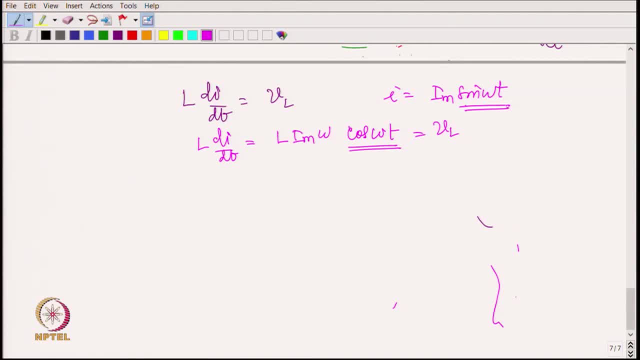 wave always leads the sine wave by 90 degrees. So I am going to have this voltage leading the current by 90 degrees. it is going to lead by 90 degrees. So if I draw the two quantities here I should probably show the voltage. 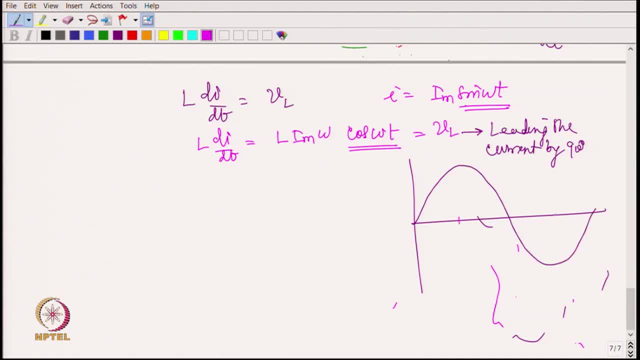 So I am going to have the voltage like this and I have to show the current as though it is 90 degrees lagging behind, like this. this is how it will be So if I try to plot both of these in the form of phasors at any instant, if I say this is what is my current, then I 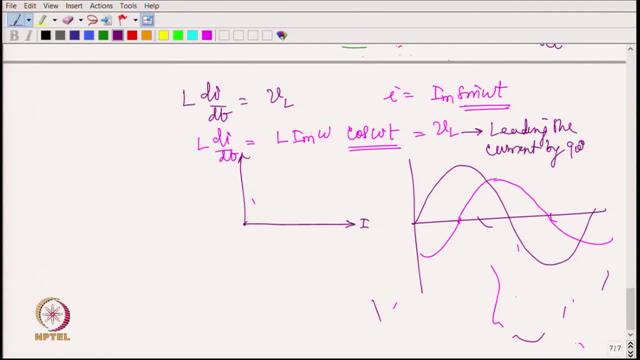 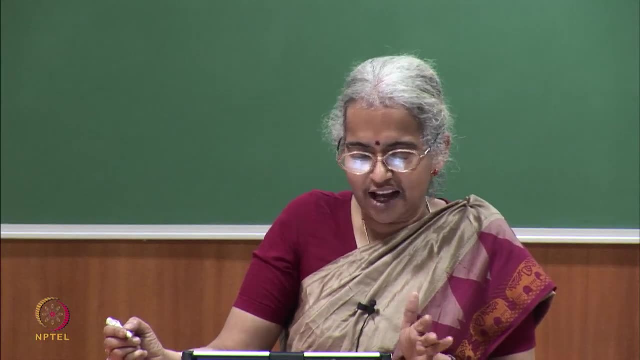 am going to have the voltage leading by 90 degrees. So this is what we call as the phasor diagram. So if I draw two of the quantities which are alternating in nature, we say at any instant of time how they are displaced from each other. So we call this as the phasor quantity. 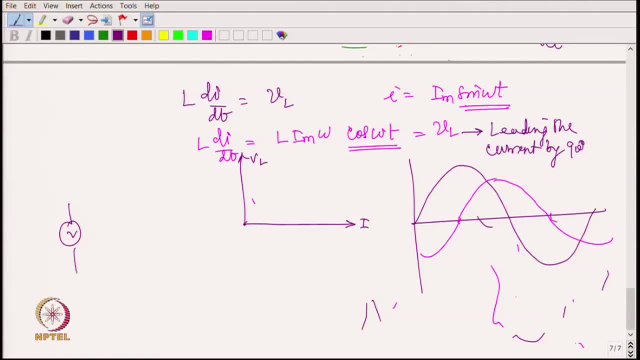 So if I have a circuit, for example, that I am going to have an alternating voltage, then may be a resistance, may be an inductance, another resistance, may be a capacitance and another resistance. It is not going to be very easy for me to draw for each of them. 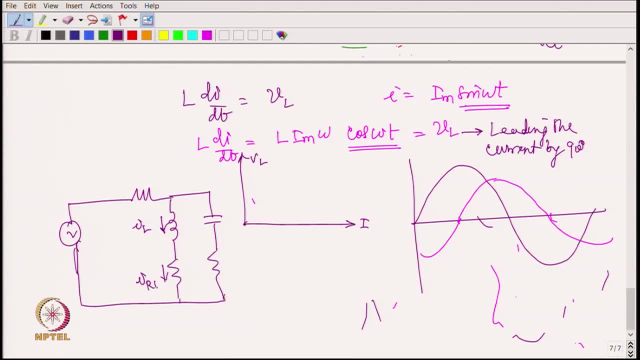 let us say So: let me call this as IL, I call this as IR1 and I call this as IR2, let me call this as may be I through C, and let me call this as IR3, and when I add these, that is these: 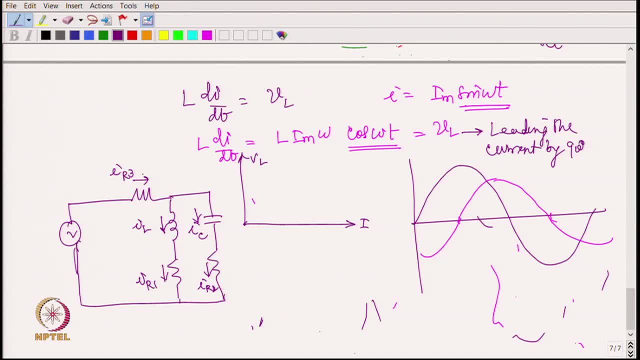 two currents I will be able to get what is IR3 and when I add, the voltage drops across these two elements and this element I will be able to get what is the voltage source. But it is not going to be easy for me, So it is going to be very difficult for me to draw all these phasors and add them. So 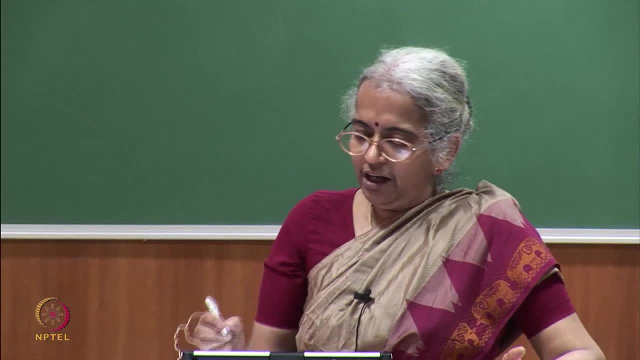 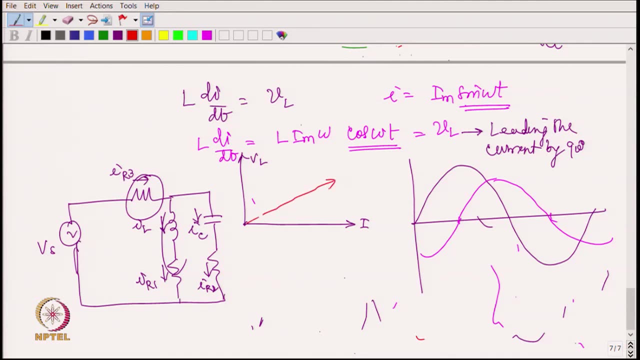 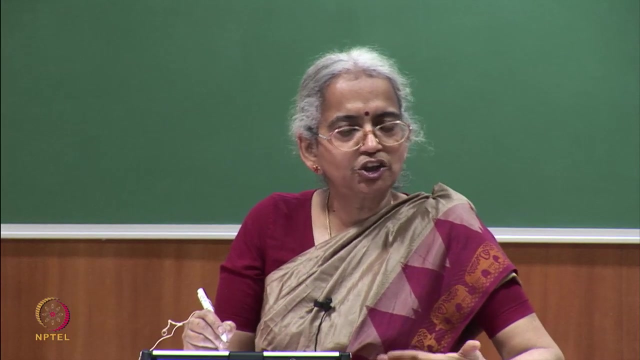 people wanted to find out what is the easier way out. Because you are mentioning voltages, and currents may be another voltage. something is here. I may mention the voltage like this: Why can't I mention this in the form of complex numbers? that is the thought that came into. 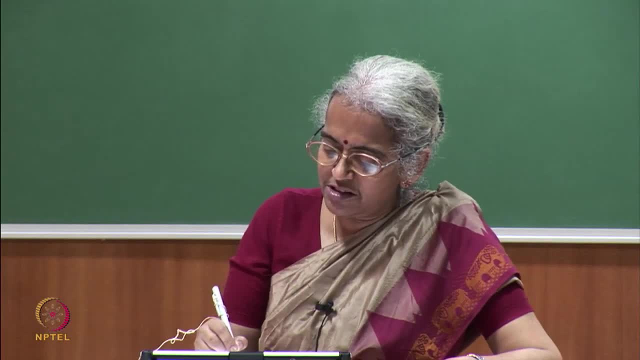 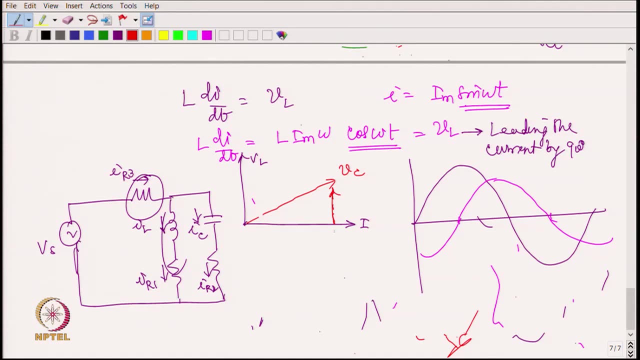 people's mind. So that is the reason why, if I say this is some VC or something, it can have a horizontal connection. Sorry, No, Can't, No, No, No, No, No, No, No. It can have a vertical component, the horizontal component we call as the real part of the 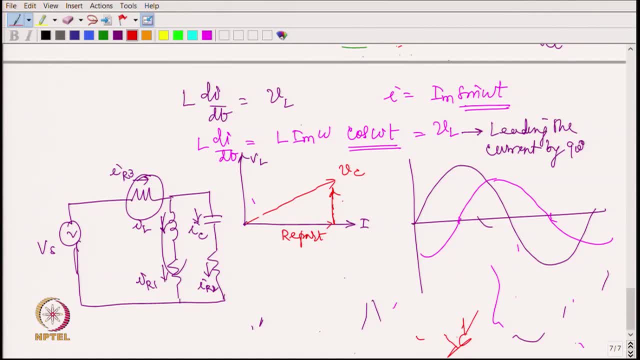 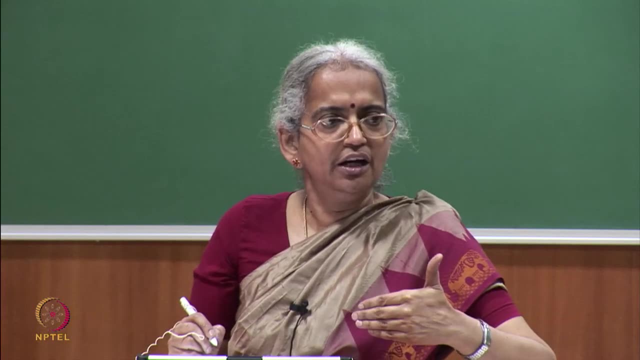 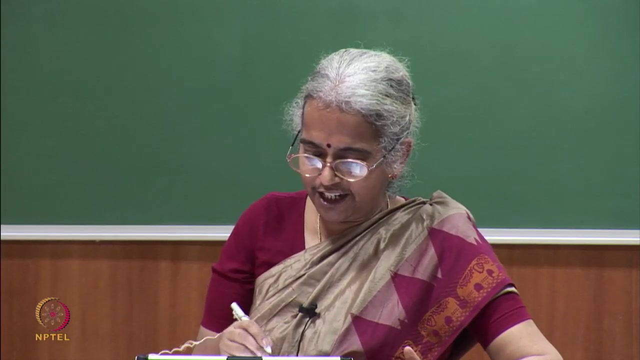 complex number and the vertical component we call as the imaginary part of the complex number, imaginary part of the complex number. So we are essentially now diversifying from mentioning a sinusoidal quantity as a phasor to indicating that as a complex number. So the complex notation mainly gives us major advantages. 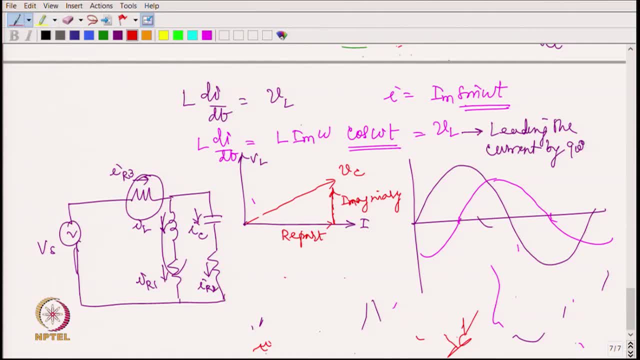 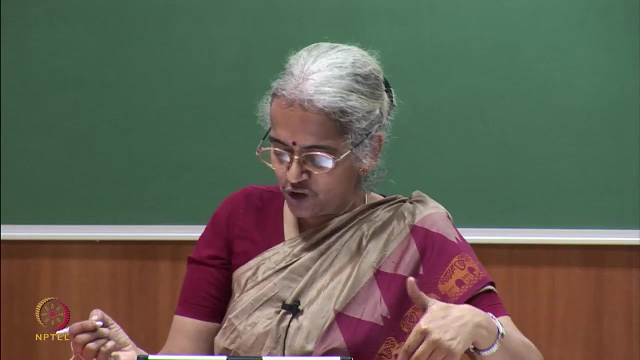 If I say, for example, il, il is going to be some a plus jb and let us say I am going to have ic as some c plus jd. please note I am not using i here. normally in complex number we use a plus ib and c plus id, but i we use normally for current. so I am using j. 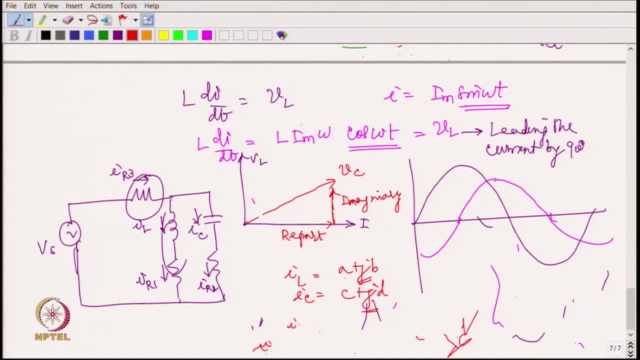 So a plus jb. So i can say il plus ic will give me what is ir3, it will be very easy for me to add it. I can say a plus c plus j times b plus d, very easy to add. So whenever we have a complex notation, the algebraic operations become much simpler. 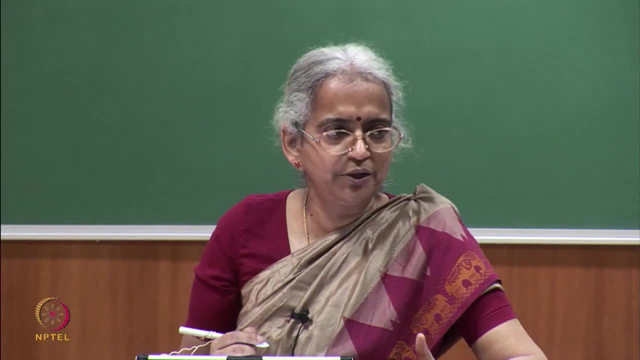 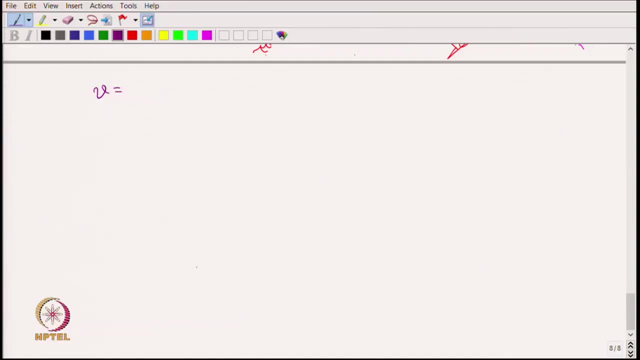 that is the reason why we have chosen to have the complex number notation, right. So once we have complex number, Let us say I have v equal to a plus jb. and let us say I have i equal to c plus jd. okay, I may be able to mention this as some v angle theta1 and I may be able to mention this as: 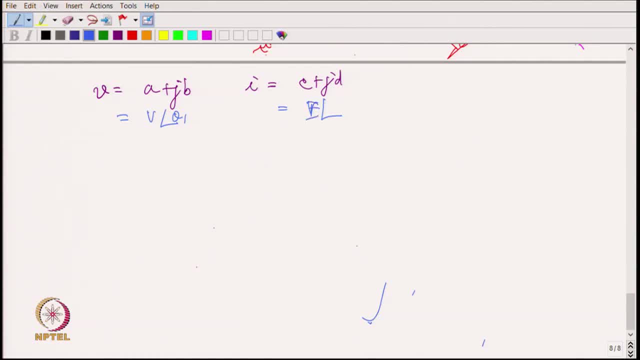 v angle. i angle- sorry, let me just erase this So v angle theta1 and i angle theta2, right. All of you know. basically, when we look at the power, we generally say vi, theta1 minus theta2 angle. this is what happens to be normally the power right. 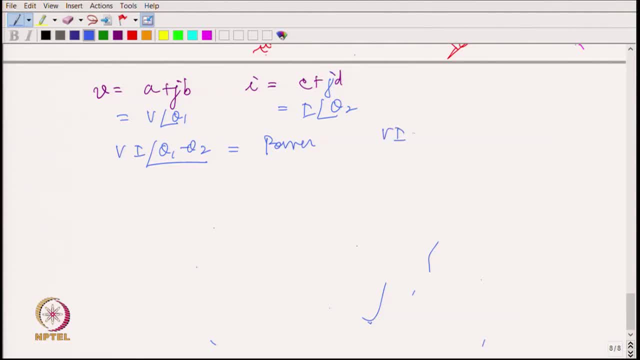 This is what we normally write as the power. what I mean is vi cos of theta1 minus theta2 will be real power. This is what you must have written. Okay, This is what you must have learnt in circuits, AC circuits. Similarly, vi sin of theta1 minus theta2 will be the reactive power. 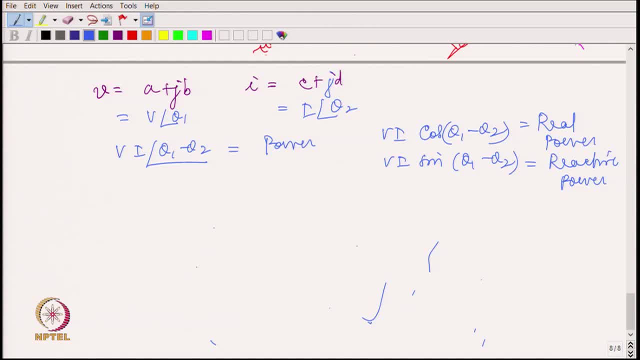 So if I want actually how to calculate this power in the complex form, let me call this as p, let me call this as q and ultimately, what I want is p plus jq. this is what I want. So if I have to write this, I have to write this as vi: cos of theta1, cos theta2 plus sin. 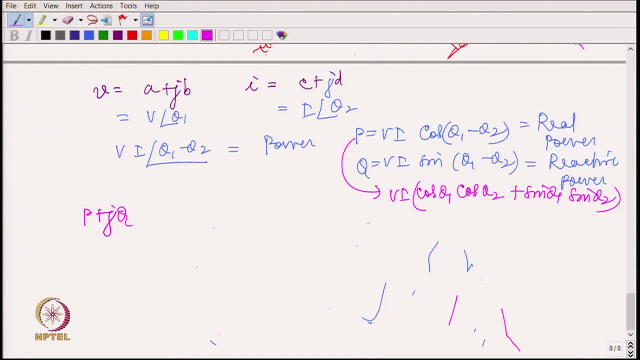 theta1 sin theta2, right. And similarly, q will be vi sin theta1 cos theta2, minus cos theta1 sin theta2.. So, finally, when I get the power which is active, Okay, Okay, So actually we call that as apparent power. 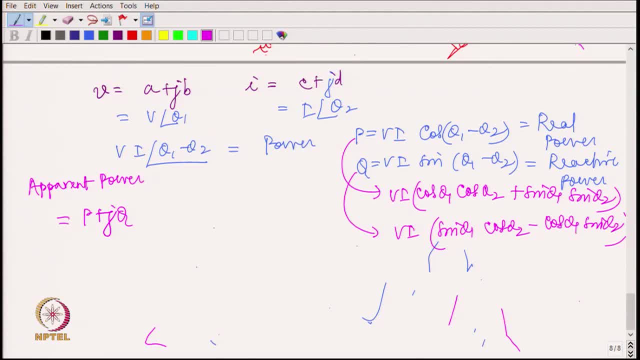 So we want to get the apparent power in the format of p plus jq. So if I actually try to do it as vi angle theta1 multiplied by i angle theta2, it is not going to work properly. So I have to take the conjugate of this particular i. if you try to calculate backwards, you 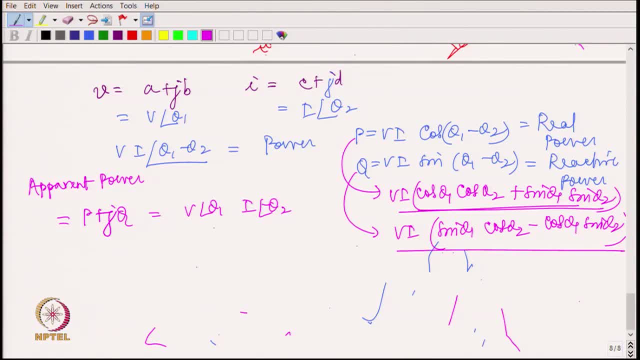 will see that you are getting this expression for p and this expression for q. So you are going to have basically, in this particular case, if I write this as vi conjugate, which means I am going to have v cos theta1 plus j sin theta1, Euler's formula I am using. 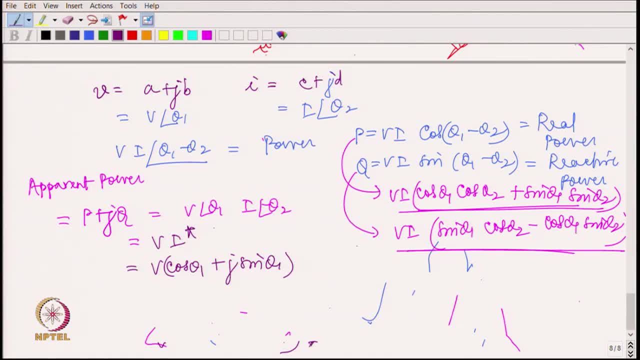 directly. Okay, Okay. So I am going to multiply i and I should say I conjugate, so it will be cos theta2 minus j sin theta2, right? So when you multiply you are going to get vi commonly cos theta1 multiplied by cos theta2. 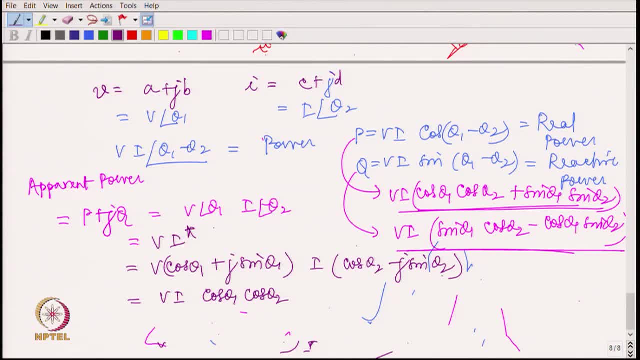 and j sin theta1 multiplied by minus j sin theta2, j multiplied by j is j square, which is minus 1, so I will get plus sin theta1, sin theta2.. So this becomes my real part, which is corresponding to the real power, and I am going to have the 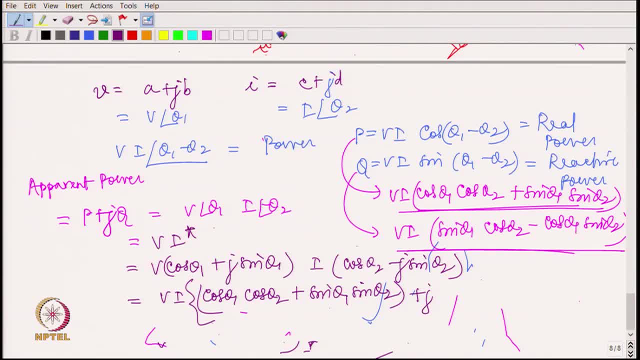 imaginary part which is going to have j. so j sin theta1 cos theta2 and I am going to have minus of sin theta2 cos theta1.. Okay, So you can see very clearly that these two are matching each other. If I look at p and q expressions that I have got, they are exactly matching with this. 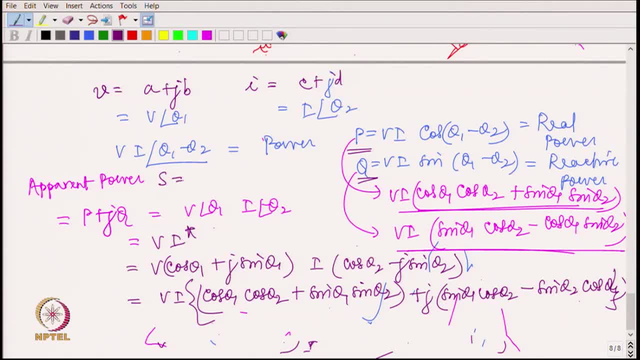 So normally we write the apparent power expression S as either vi conjugate, iv conjugate and so on, So we can have one of them conjugate. that is what is important. So complex notation gives us an very easy way for calculating power. calculating power. 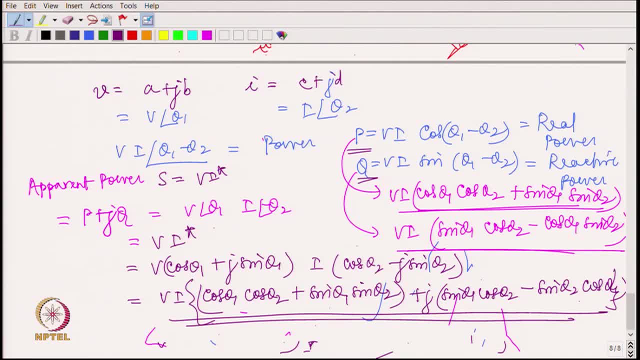 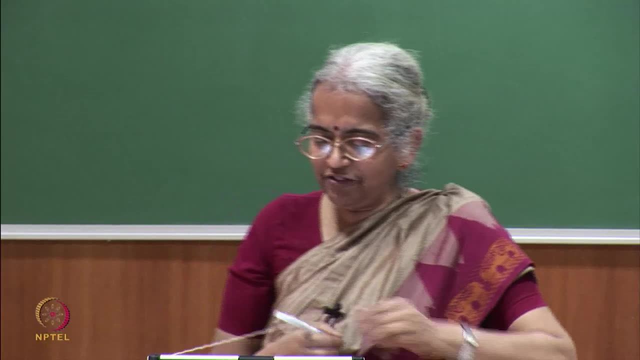 Okay, Okay. So calculating summation of currents or multiplication of currents, multiplication of voltages and so on, All those things are done quite easily when we have complex notation, right? So, in general, single-phase quantities, when we look at single-phase AC quantities or single-phase, 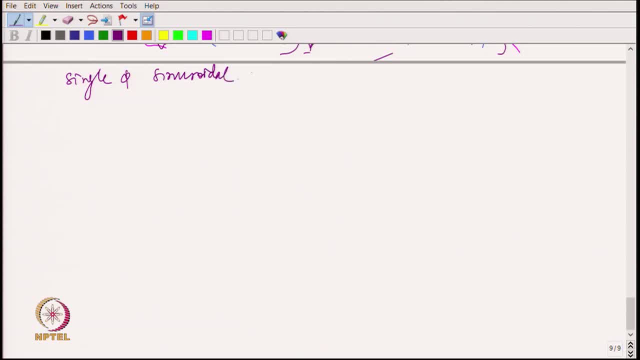 sinusoidal AC quantities. They are represented mainly in two forms. Okay, One is in complex form and the complex form indicated is also indirectly translating into phasor diagram. So we will be repeatedly using these for getting our power. or phasor diagram equivalent circuit. 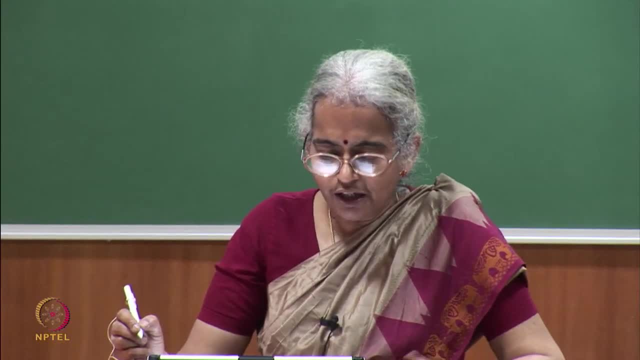 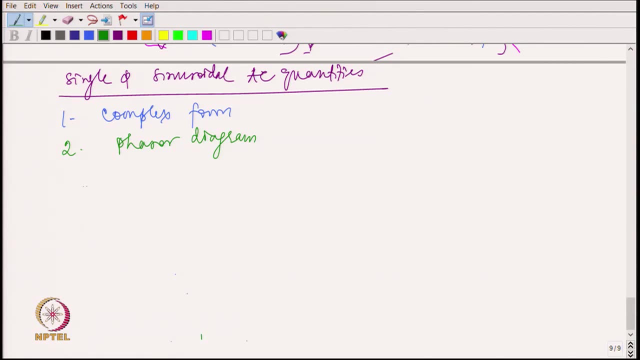 all of them in transformers, AC machines and so on. So this is really important to know. Now let us recall the following. Let us recall some of the principles corresponding to three-phase circuits. So if you look at many of the electrical machines that are available in the market- AC machines- 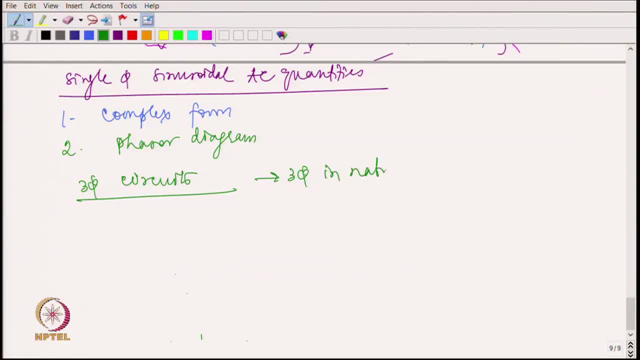 they are all three-phase in nature. This was initially actually the three-phase configuration was initially introduced by Tesla. It was invented by Tesla And he had made the induction circuit. This is the induction circuit. Okay, He had made the induction motor sometime in 1890s or something. 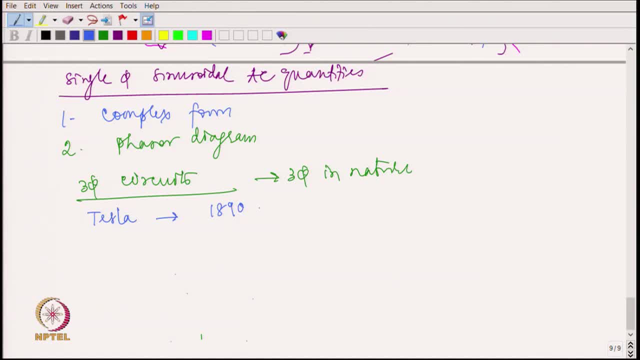 So induction motor design has not changed until date. It is almost remaining the same ever since 1890.. So if you actually look at the three-phase, the major advantages, if I look at the advantages of three-phase, because I have in three-phase I am going to have Va, Vb, Vc and in all the 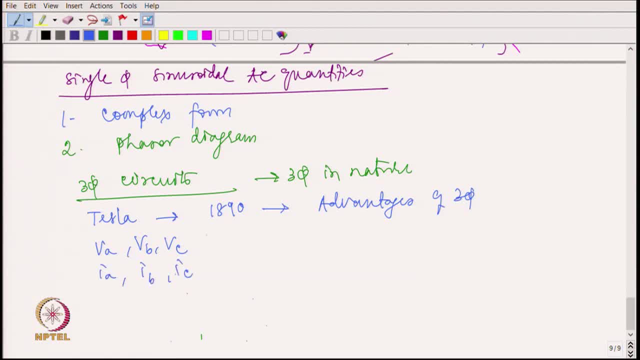 three-phase circuits. I am going to have Ia, Ib and Ic and the overall power is going to be Va, Ia plus Vb, Ib plus Vc, Ic. this is going to be the power, So if one of them is low, the other one may be high. 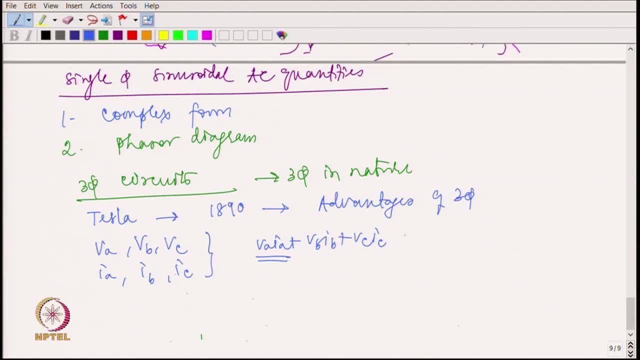 So all of them balance with each other and ultimately you get a constant power or constant torque. ultimately. So if I say constant power, power divided by omega is going to be torque- Not in any rotating machine. So the torque also becomes a constant quantity, roughly. 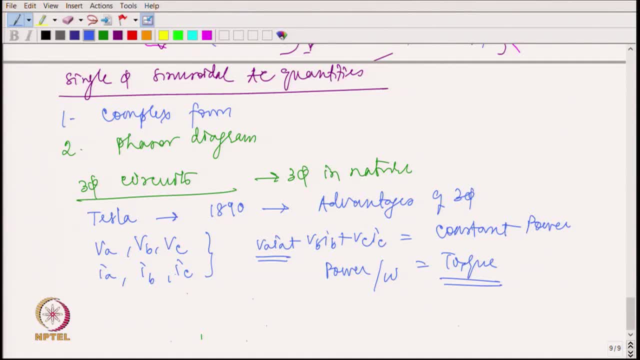 Because you have the power and torque to be constant, it is very suitable for high capacity applications. What I mean is megawatt level applications or even hundreds of kilowatt level applications. You do not want the torque to change continuously. If the torque changes continuously, you are going to have vibrations in the shaft, which 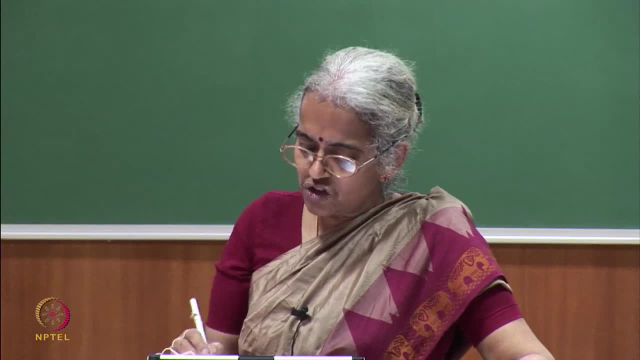 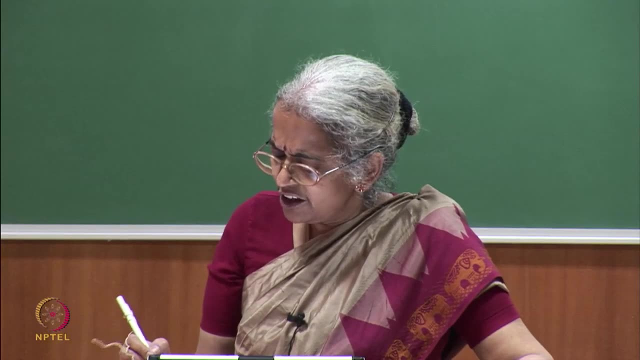 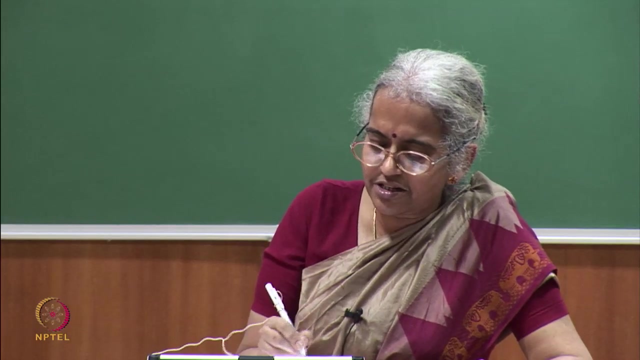 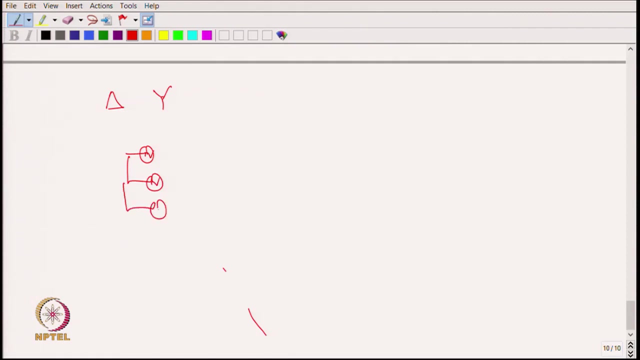 cannot be tolerated, Especially at high capacity. So three-phase is really really good for high capacity applications. And one more thing is that I am sure you guys know that three-phase can be connected either in star or delta. So if I have Va, Vb and Vc- all the three-phase voltages- they can be applied to either star. 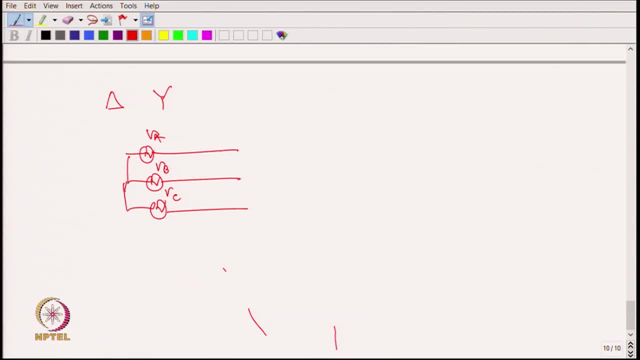 connected circuit or delta connected circuit. So, throughout, if I look at the transmission lines that are going, I can just have three transmission lines. That is it, And I will be able to disseminate power, which is three times single-phase power, Whereas if I am disseminating the whole thing in the form of single-phase power, I am essentially 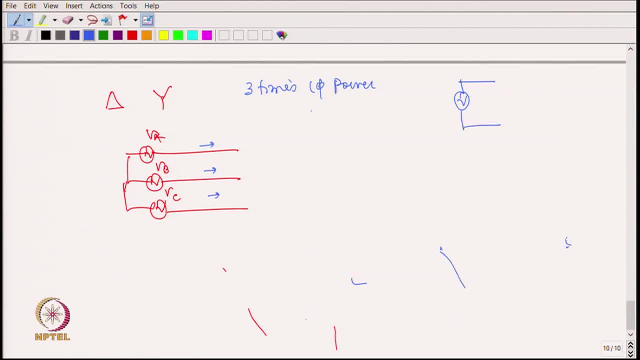 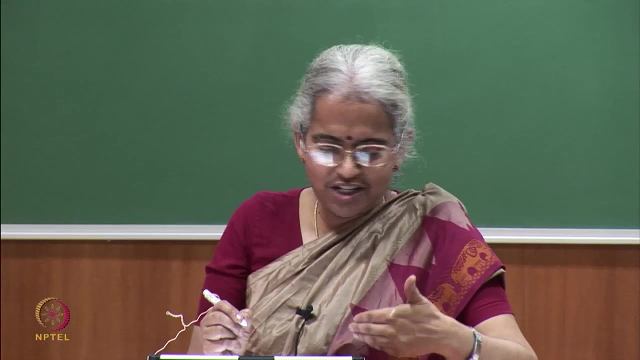 going to require two conductors for disseminating just P, Whereas here I am disseminating the three P for which I require only three conductors. So the cost, what is involved in copper conductors, that comes down drastically when you go from single-phase to three-phase. 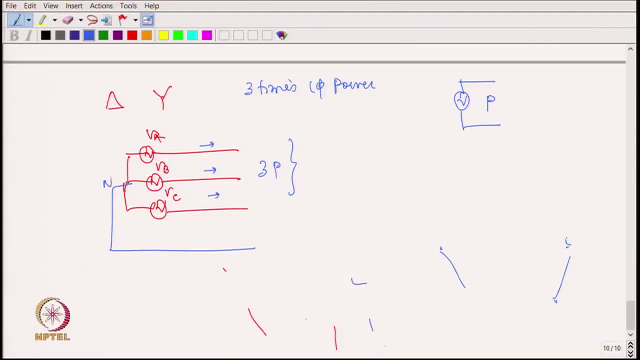 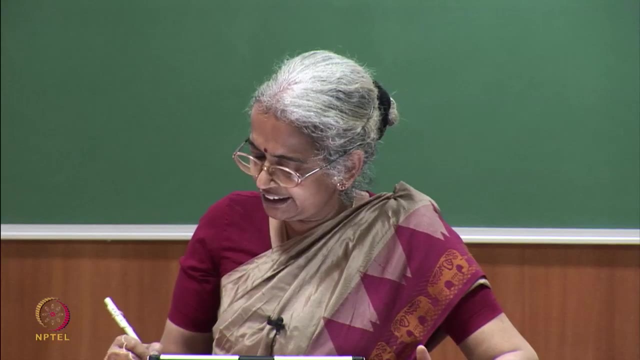 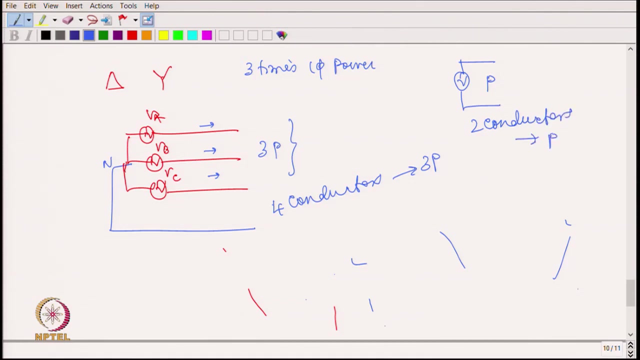 Of course, in most of the cases we will be having a neutral conductor. also, If you look at most of the transmission lines, we will be having a neutral conductor. So even then, four conductors are able to transmit three P, Okay, Whereas here two conductors, two conductors, are transmitting only P. So obviously we are. 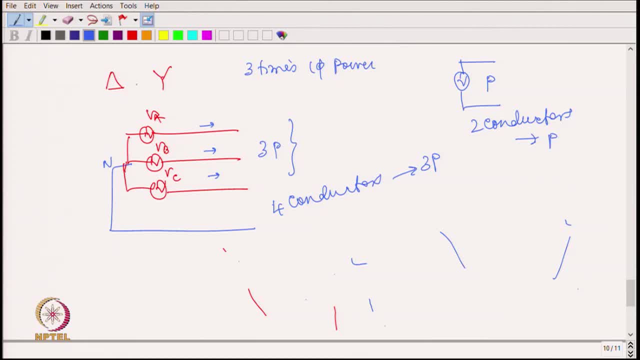 saving on the cost of copper. So three-phase is very, very commonly used for generation, transmission as well as distribution, except for domestic application, Only for domestic application. we are going to use single-phase right. So it is very important to learn about three-phase quantities. 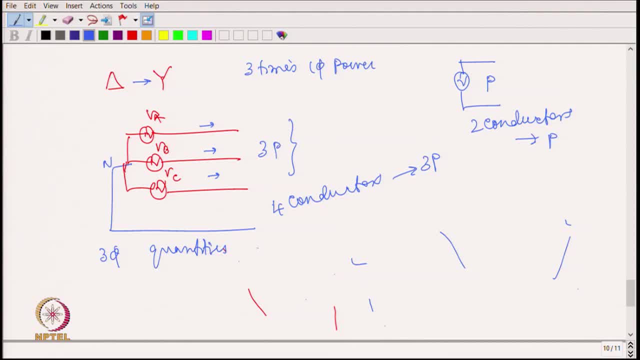 Okay, So that is how we measure power and how we are going to actually justify measuring the power and reactive power. So how we are going to measure these things. that is what we are going to see next. So we are going to look at three-phase power measurement. 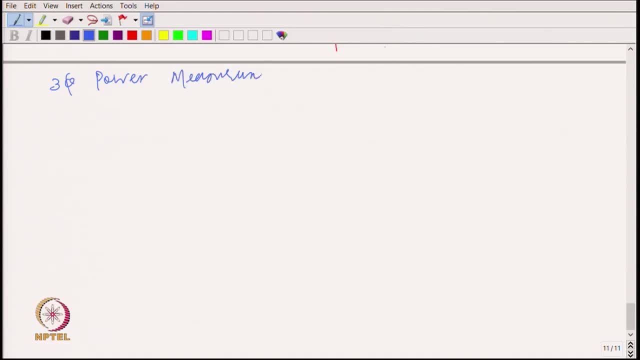 If it is balanced load. I am not going to take the case of unbalanced load condition Because most of the electrical machines normally are balanced, So there is no need to really talk about unbalance. There are different power measurement methods. It can be with single wattmeter, but this can work only if neutral is available. 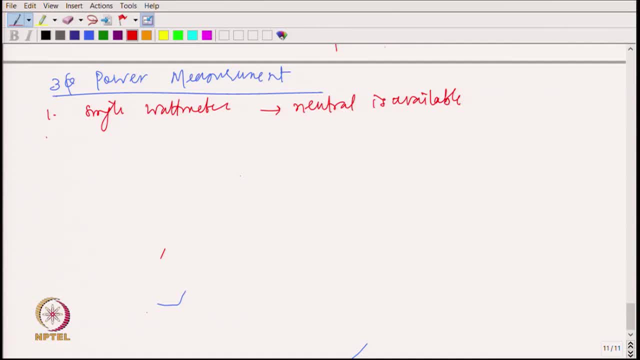 Most of the times, neutral may not be available, So we may not be using it. Similarly, three-wattmeter method- Okay, Okay, Okay, Which will also be used only if the neutral is available. otherwise it is not going to be easy. 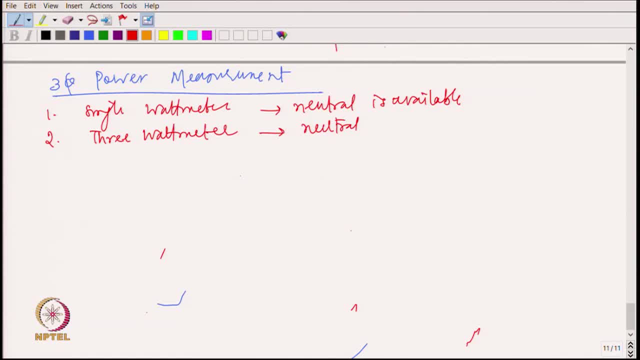 If it is delta connected, we can still think of using this, probably three-wattmeter method, but two-wattmeter method is a very, very common method which is used for using used for measuring power in a three-phase balanced as well as unbalanced system. 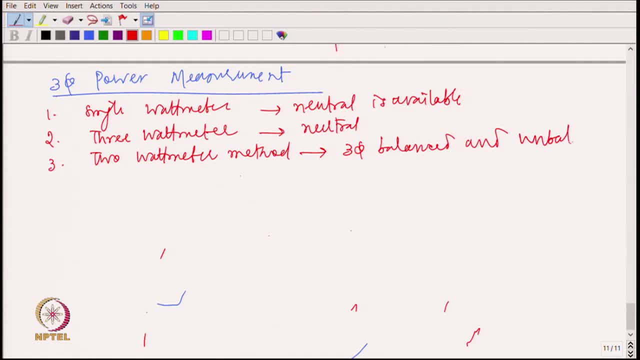 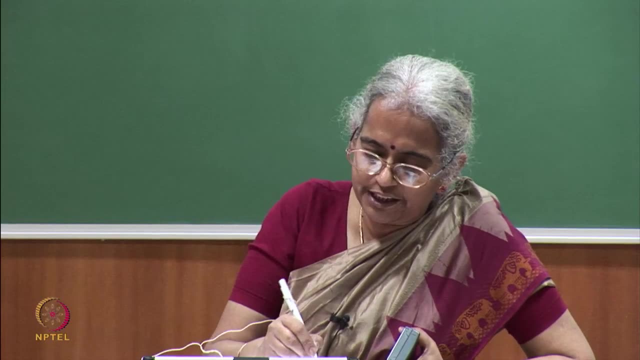 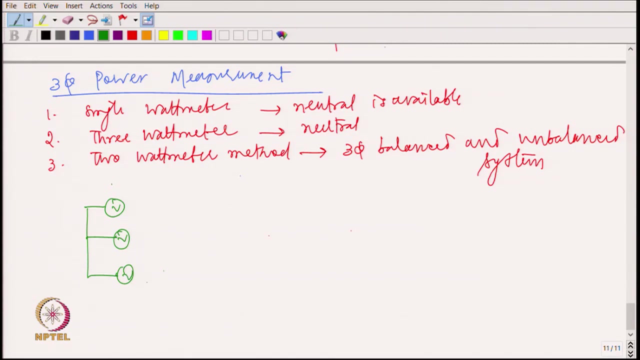 Okay, Okay. In both the cases it will work quite well. So what is this method all about? That is what we are going to see now. So let me draw the circuit diagram corresponding to the two-wattmeter method. Let us say I have a three-phase supply here. 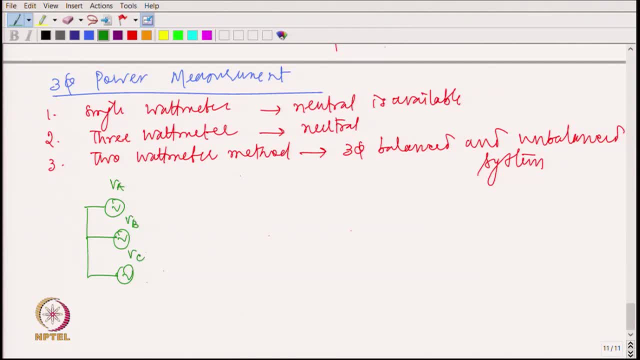 So let me call this as Va, this is Vb and this is Vc and this is the neutral. Okay, Now I am going to have probably a load here. The load can be delta connected or star connected, So I am showing the load just like a black box. 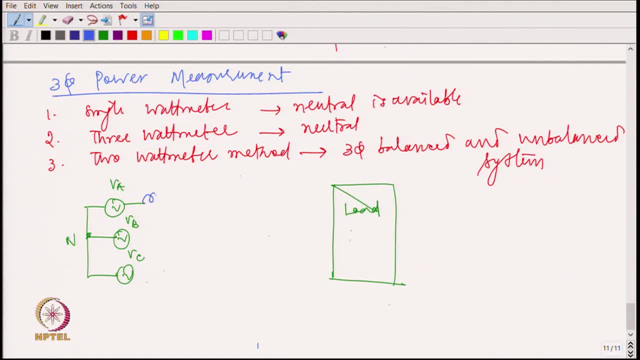 So I have only two wattmeters with me, So I am going to connect one of the wattmeter current coil here, another wattmeter current coil here And I am going to connect the voltage coil or the pressure coil like this. Okay, 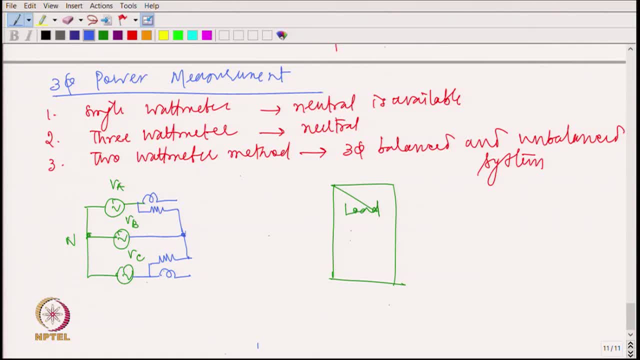 So the pressure coil is connected between the phase in which the current coils are connected and the other phase which is not having any current coil. Then this is connected directly to the load. I am sure you guys have seen already the wattmeters. So there will be the current coil which will be actually connected between M and L Normally. 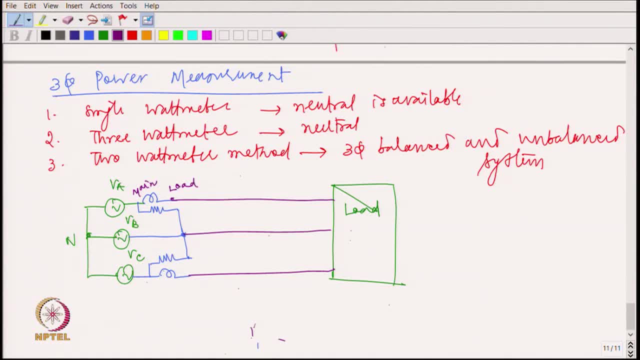 this stands for load, M stands for the mains And similarly I am going to have here also M and L. Let me call this as M1 and L1.. Okay, So this is the current coil 1 and I am going to have the pressure coil connected between. 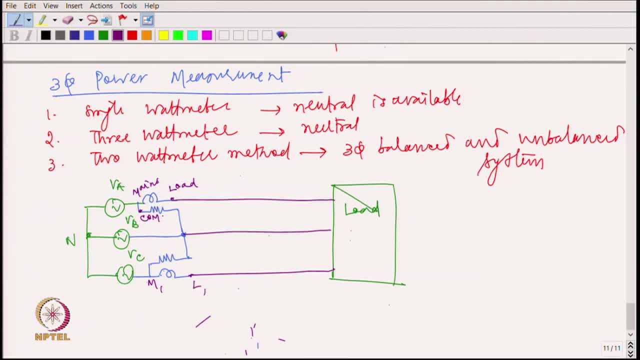 the common point which is common between the current coil and pressure coil, and this is going to be the V. So similarly, here also I am going to have common 1 and V1.. So this is the connection that we are going to have in the 3 phase 2 wattmeter matrix. 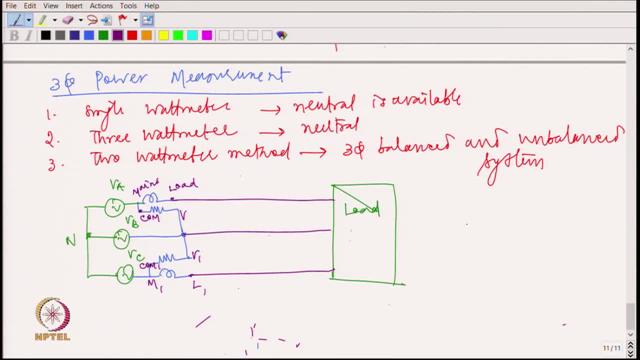 Okay, Let me first of all try to justify that. this will give me 3 phase power. So normally, if you look at the 3 phase power, you are going to have V1, I1 or Va, Ia plus Vb, Ib plus Vc, Ic. 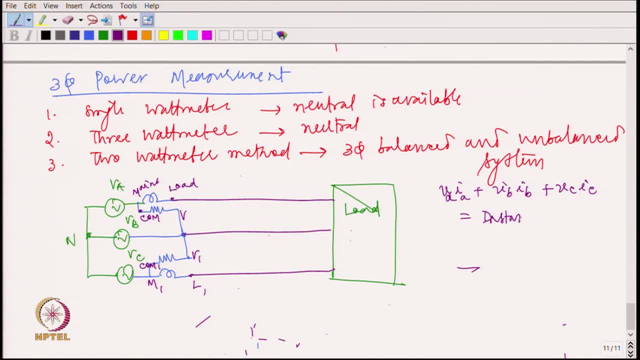 This is the instantaneous 3 phase power, right, but if I try to look at what is the actual value of power, So normally we write, we write this as P equal to root 3 VL. Il cos phi right where phi. 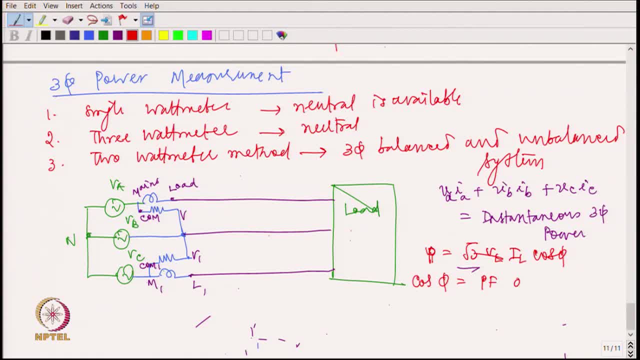 cos phi is the power factor of the load. So load power factor, I am calling as cos phi. in this particular case, this is going to be the power factor. Okay, So let us try to see 1.. So what is it that I am going to get in? wattmeter 1 and wattmeter 2 respectively. 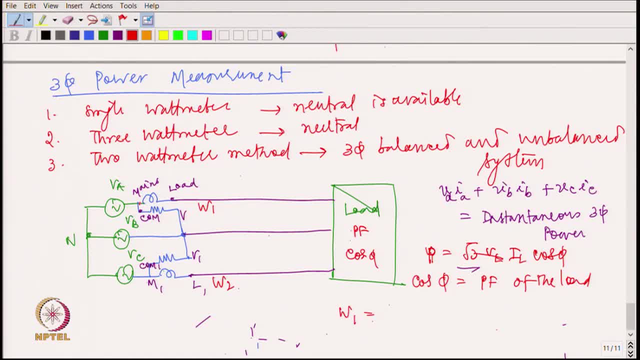 So in wattmeter 1, I have here voltage of A phase and here voltage of B phase, So I am going to get Vab as the voltage across the pressure coil of this particular wattmeter and the current through this is going to be Ia. 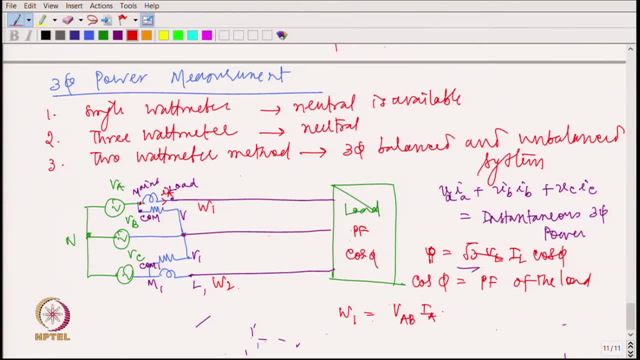 So I have to write this as Ia- Please note- I am writing RMS quantities, All of them are RMS quantities. Okay, RMS quantities. So this is Vab multiplied by Ia right and between Vab and Ia. whatever is the angle that, 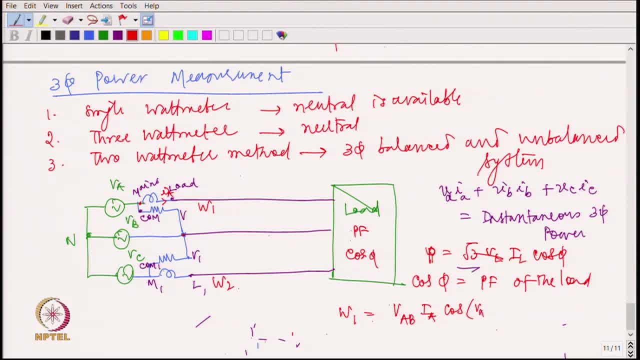 is present. I should say cos of the angle between Vab and Ia. This is going to be the reading of W1.. Similarly, W2 is going to have the reading to be: this is voltage of C and this is B, so I am going to have Vcb. 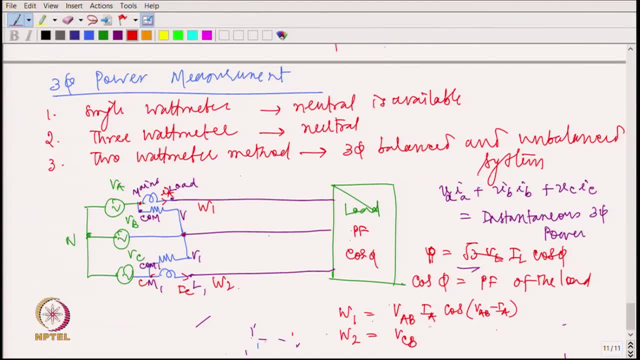 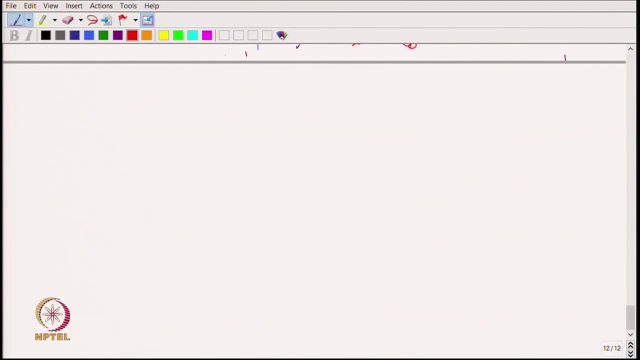 And the current that is flowing here is Ic. So this is going to be Ic, cos of Vcb and Ic. right, This is going to be W2.. So let us try to take a look at exactly how this looks when we are having the phasor diagram. 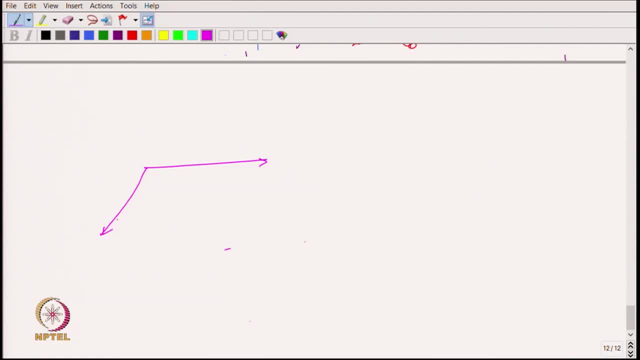 completely drawn. So let us say: this is Va, this is going to be Vb and this is going to be Vc. Okay, These are the three phase voltages. They are phase shifted from each other by 120 degrees. When I want Vab, I can take Vb on the other side. 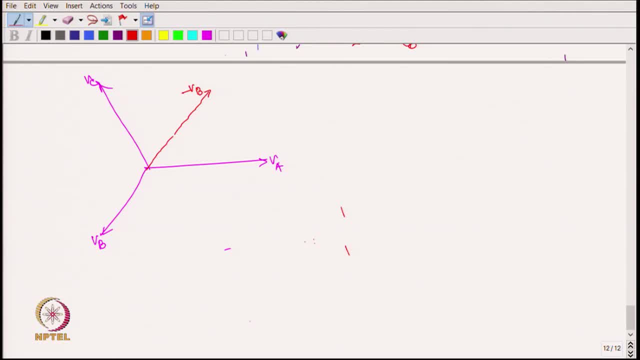 So this is actually minus Vb. So when I try to look at what is Vab, I have to just take the resultant of Va and Vb added together, So I will have this as Vab, Okay, Okay. Similarly, I should be able to draw Vac, which will be the mid in between these two. 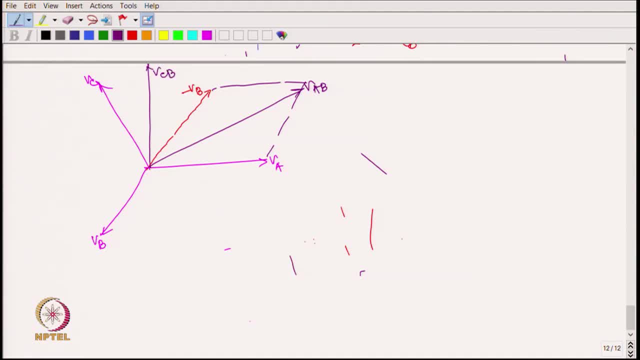 I cannot go beyond this, So this will be Vcb. Okay, Now let us say I am going to have a lagging load. I am just arbitrarily taking this as some at a power factor angle, phi, This is going to be Ia and if I assume it is a balanced load, I am going to have Ib. 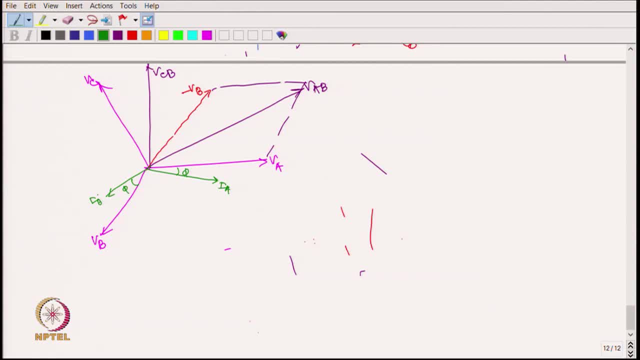 Okay, Again at an angle of phi and Ic. somewhere here, which is also at an angle of phi Right Now, I have to look at what is the angle between Vab and Ia if I want to get the power of W1.. 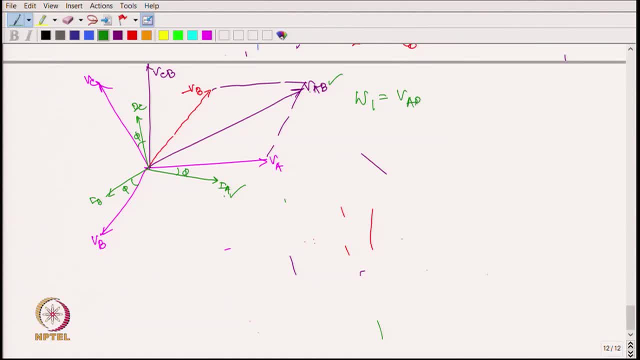 So I am going to have W1 equal to Vab Ia. This is 30 degrees, Right? So this is going to be cos of 30 degrees plus phi. Similarly, if I try to write what is W2,, W2 is going to be Vcb Ic, but this angle is again. 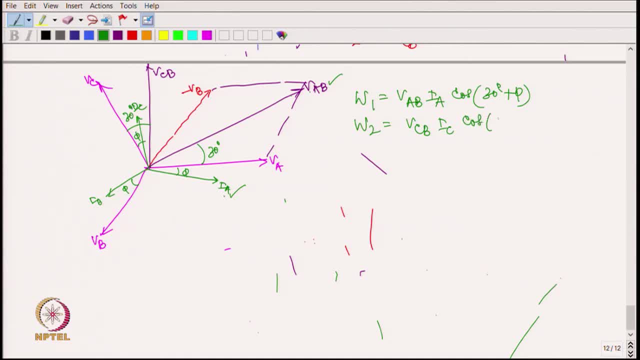 30 degrees. So I am going to have cos of 30 degrees minus phi, Right, So I am going to have, When I calculate, W1.. W1 plus W2 it will be Vab or Vcb. I can call them as line voltage, Vl directly. 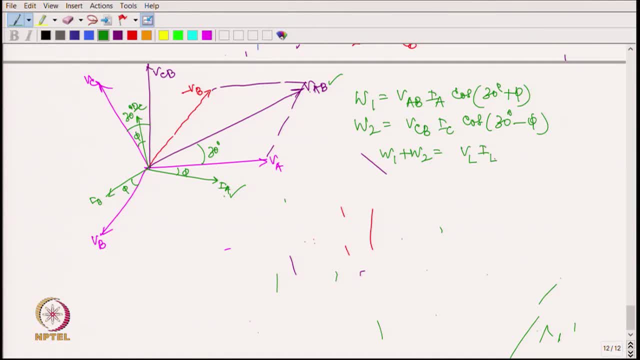 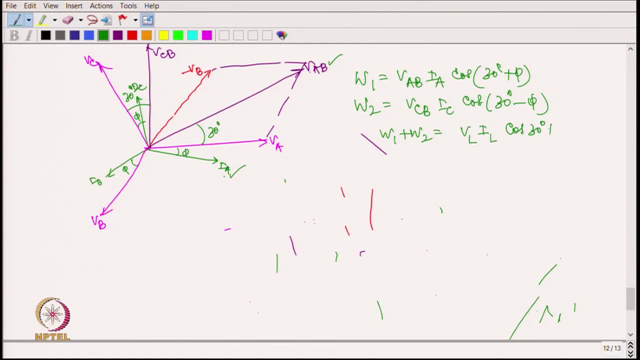 Similarly, I can say Ia or Ic. if it is a balanced load condition, I can call that as Il and I can say: this is cos of 30 plus phi plus cos of 30 minus Vc. Okay, Okay, Okay, Okay. 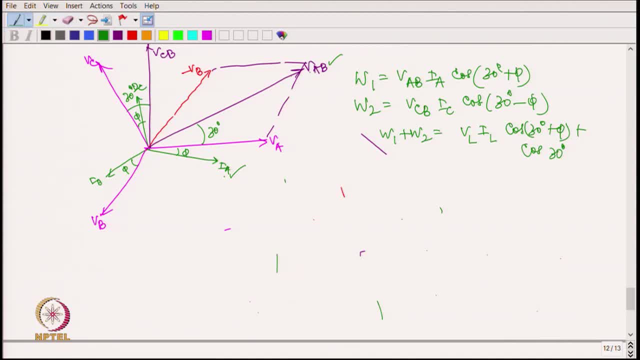 Okay, So this is going to be Vl Il cos. cos is actually going to be cos of 30 and cos of phi. Cos of 30 is root 3 and we are going to have 2 times Right: 2 cos 30, cos phi. 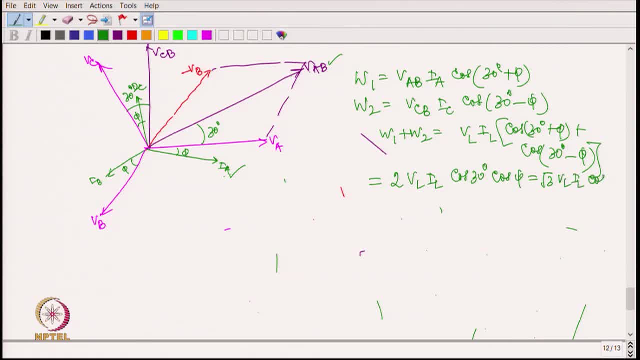 So this is going to be root 3 Vl Il cos of theta. Okay, Okay, Okay, Okay, Okay, Okay, Okay, Because cos 30 is root 3 by 2.. So we wrote the power expression earlier as root 3 Vl Il cos phi. 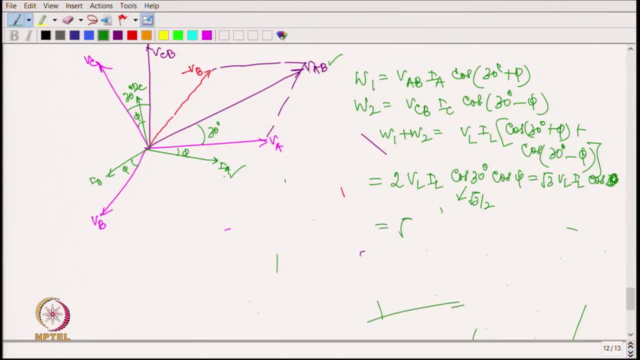 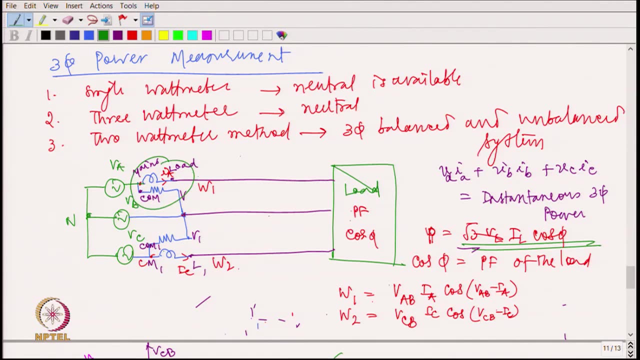 We are having essentially the same thing: root 3 Vl, Il cos phi coming out as W1 plus W2.. So this is essentially the 3-phase power expression. So we are able to measure the 3-phase power just by using 2 wattmeters. 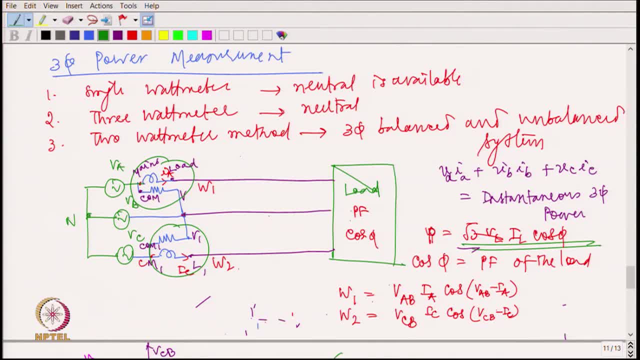 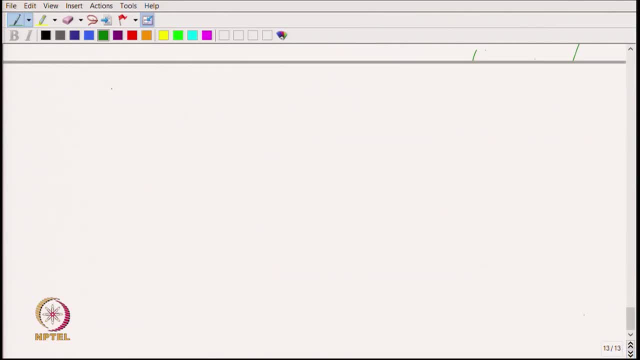 Okay, And this is one of the most reliable methods as far as the 3-phase system is concerned. But we wrote V1 equal to Vl Il cos of 30 plus phi, and W2 we wrote as Vl Il cos of 30 minus. 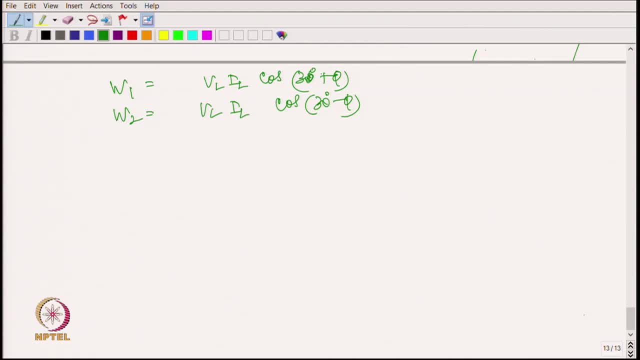 phi, Okay, Okay, Okay. So this angle happens to be greater than 60 degrees. Very clearly, I am going to have this to be cos of 90 or greater than cos of 90. So if the power factor angle happens to be 60, I will have one of the wattmeter readings. 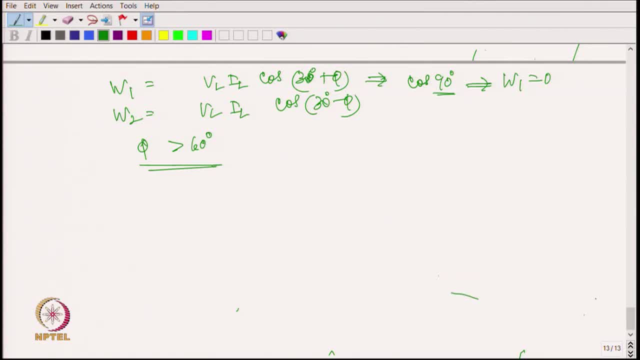 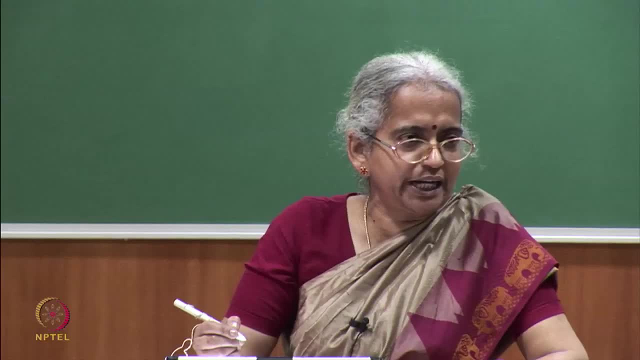 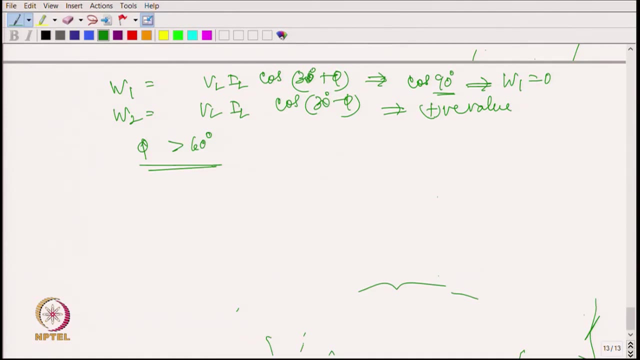 to be 0 and the other wattmeter reading will have a value which is positive, because 30 minus whatever is the angle, cos of theta equal to cos of minus theta. So I will have a positive value, Whereas if I am going to have the power factor angle to be greater than 60, W1 will be negative. 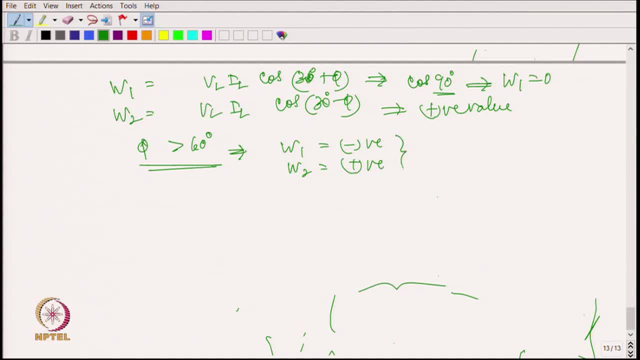 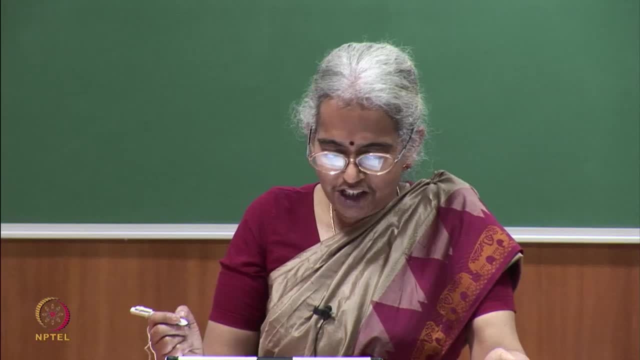 and W2 is going to be positive. That is why you will see that in some of the 3-phase experiments, when you do, one of the wattmeters might be kicking back, So in which case, if you try to reverse either the voltage or the current, you will be able. 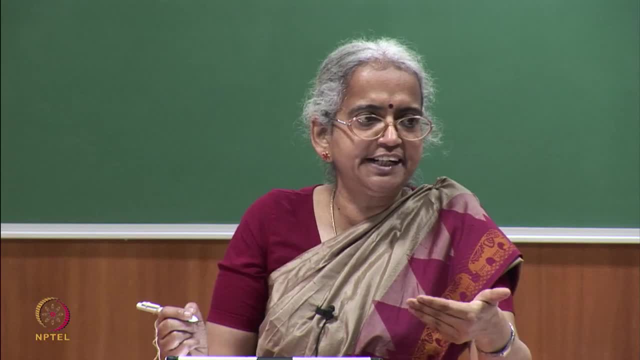 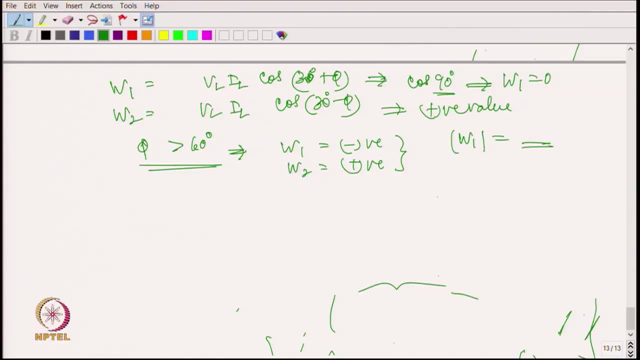 to get a positive reading But that you have to treat it as a negative value and subtract it. You cannot. in that case you have to say W1, magnitude. whatever you get is some value X, Whereas W2 is going to be a positive value. let us say Y, then you are going to say Y. 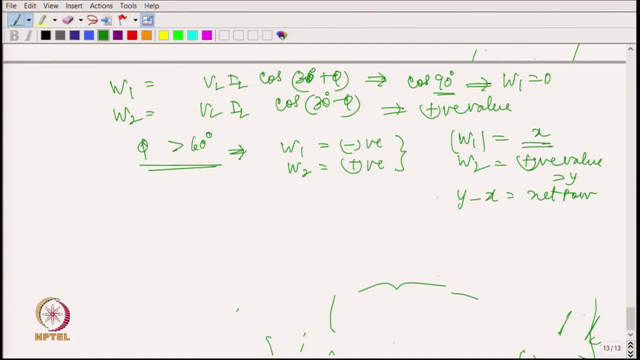 minus X is the net power in that particular case, Right. Similarly, if I get W1 equal to W2 by chance, Right, I am going to have essentially W1 plus W2 as the total power, no doubt. But I can also say from these 2 expressions, because I am having W1 to be VL, IL, cos 30 plus. 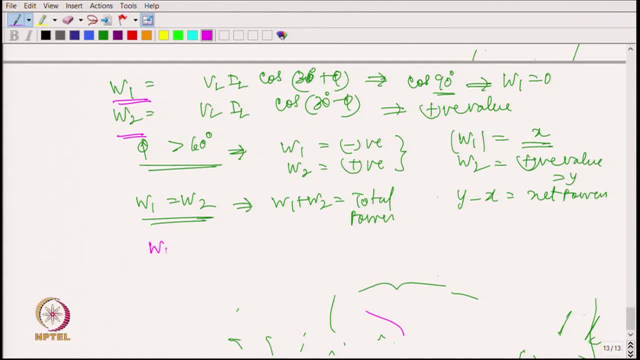 5 and W2 to be VL IL cos 30 minus 5, W1 minus W2. I can write this as VL IL cos of 30 plus 5 minus cos of 30 minus 5.. And I can write this as VL IL cos sin of 30 and sin of 5.. 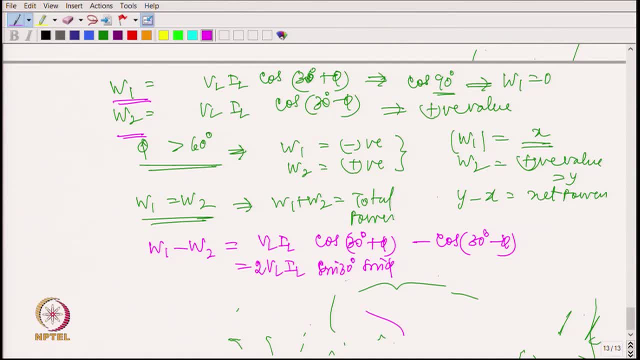 Right, Sin 30 is half. so I am going to get basically VL, IL sin 5.. So if I try to write what is sin 5 divided by cos 5. Right, That will be W1 minus W2 divided by W1 plus W2, I will get sin 5 by root 3, cos 5.. 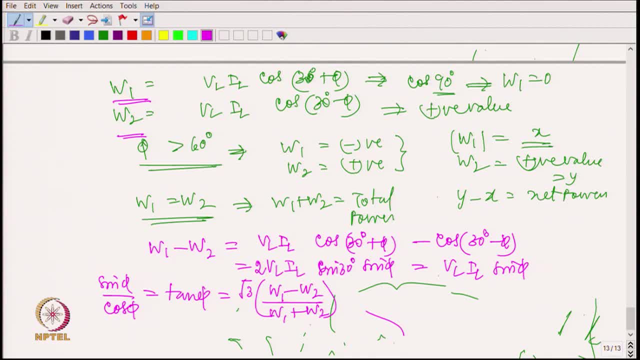 So I have to multiply this by root 3. This will give me tan 5.. So if W1 equal to W2, then tan 5 is going to be 0. From here I can say tan 5 is 0, which means it is going to be unity power factor condition. 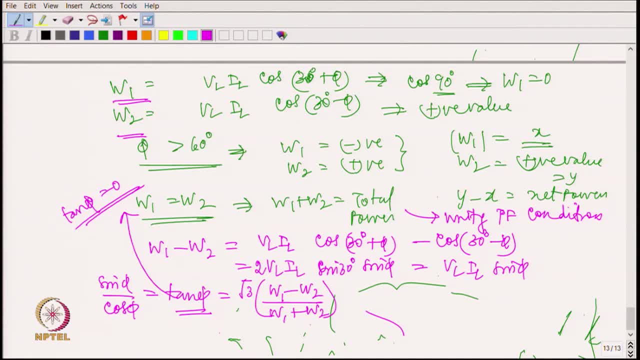 When W1 equal to W2, it will be unity power factor condition, So we would be able to deduce the power factor of the load. if I have these 2 readings with me- W1 and W2,- these 2 readings with me.